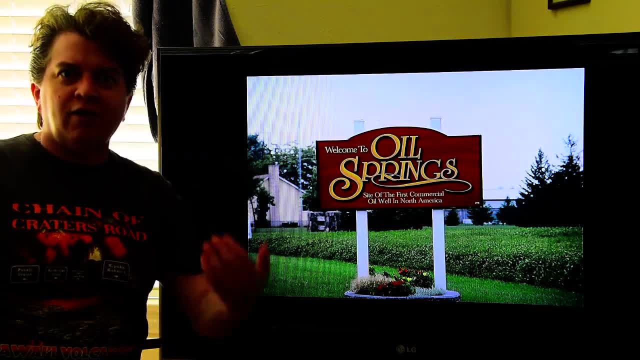 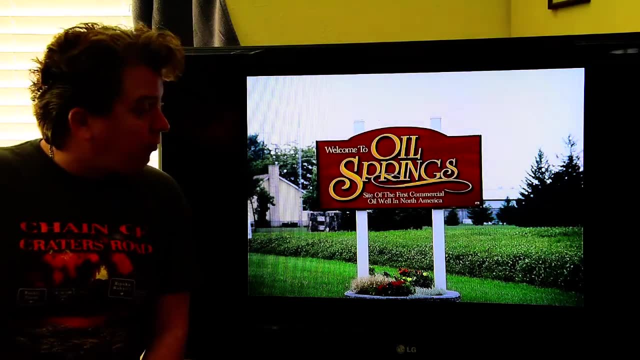 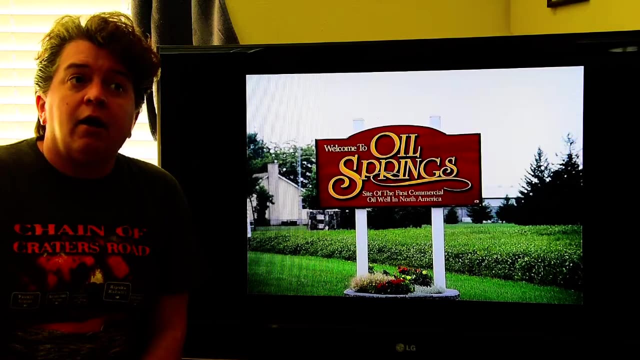 when we're watching YouTube videos, said it's Oil Springs Ontario, Of course, Right, All right. this really is Oil Springs Ontario, site of the first commercial oil well in North America. The first commercial oil well in the United States was in Pennsylvania, The 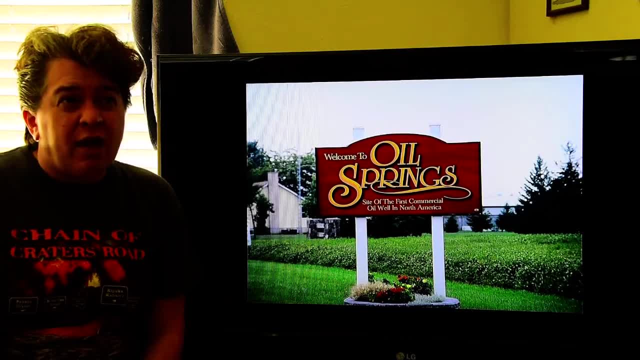 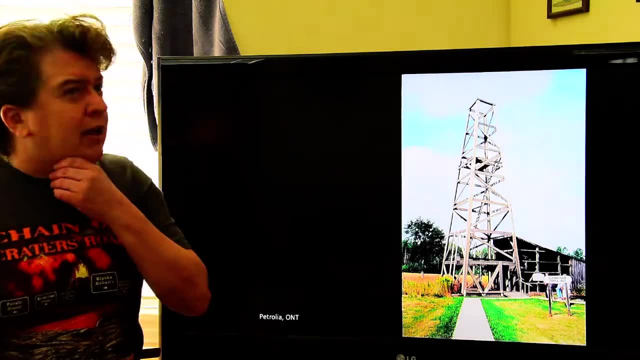 first commercial oil well in the United States was in Pennsylvania And this is the site of the first commercial oil well in the world. I think was in Azerbaijan, which is one of the former Soviet republics. So anyway, back in, I think it was 1858, was when the 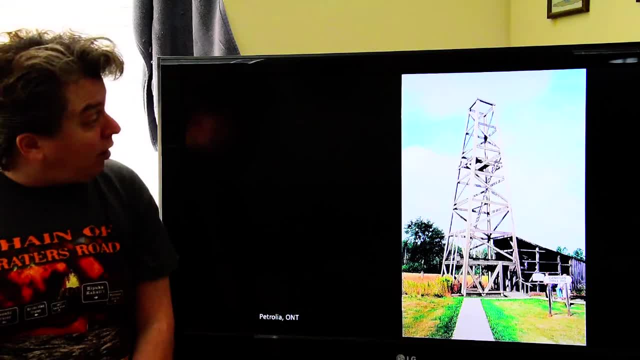 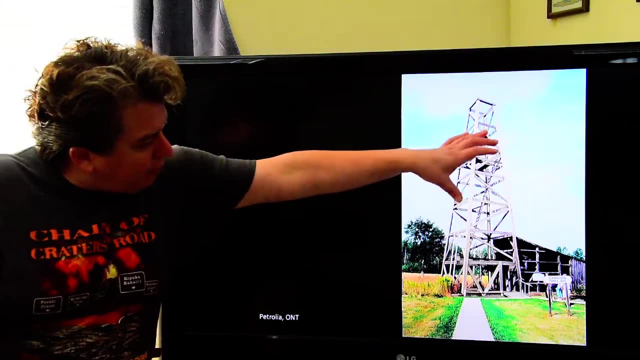 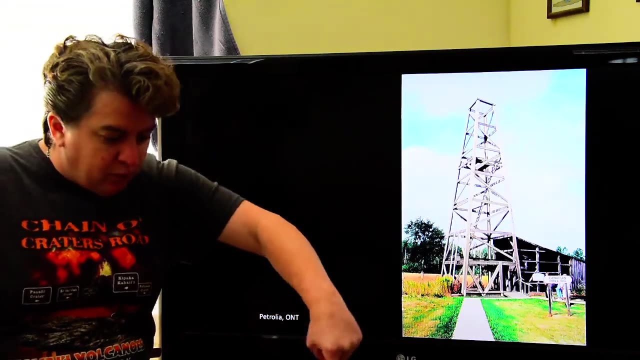 first oil well was dug And in the early days of drilling for oil they would build a rig like this And in there would be a drill that rotated And in there would be a drill that rotated And as it rotated it basically broke up the rock and drilled the oil well, And then 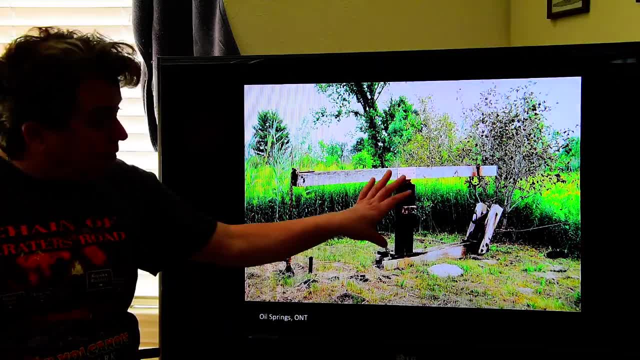 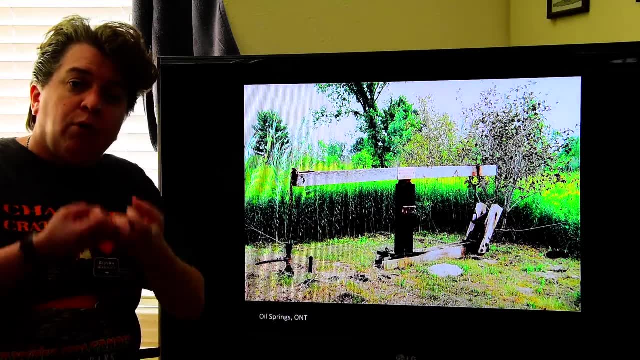 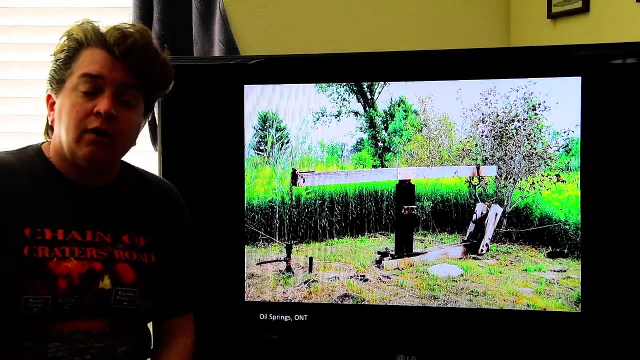 once they were done drilling the well, they would put one of these pumps on there And this pump would rock back and forth And each time it would go up it would pull some oil out And back in the 1800s this would actually run off a steam engine And the steam engine could operate. 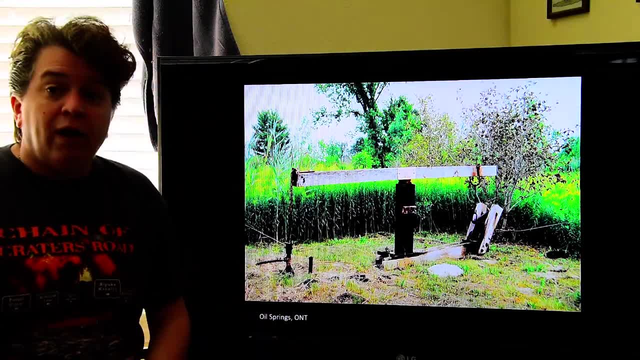 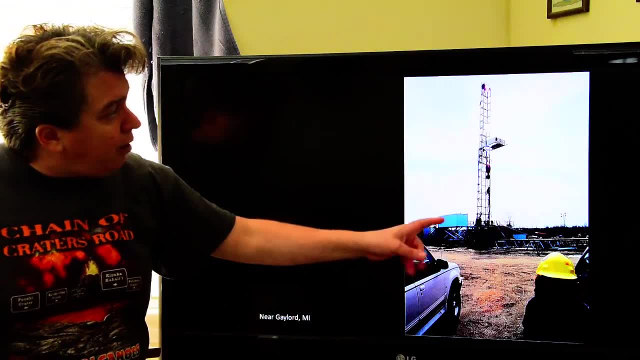 hundreds of these, of these oil wells, And this was the first oil well in the United States And we actually had this rig built and it's in a very true past. It is in a real present day oil well. Well, what do we do today? Well, today, this is a modern drilling rig set up And in there 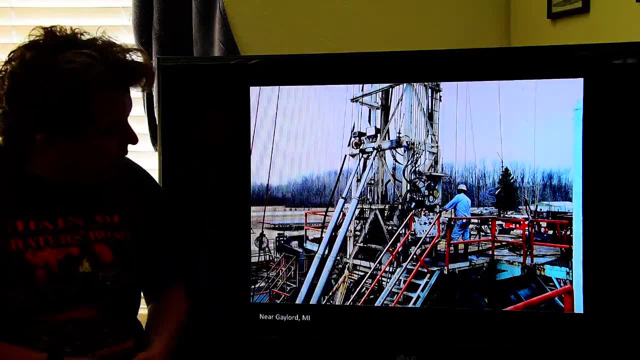 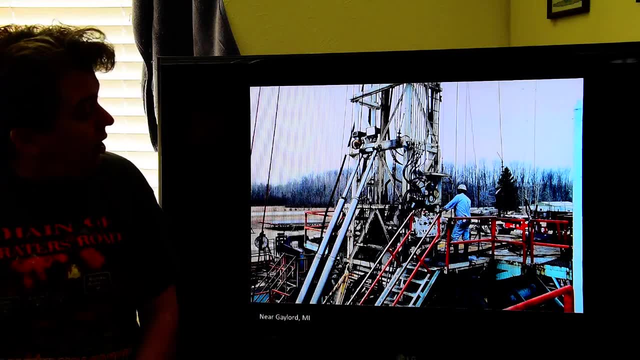 there is a drill right. It's right in there And it rotates around And as it rotates, it carves away, it chews up the rock, And that's how we drill the well, And I don't want to make 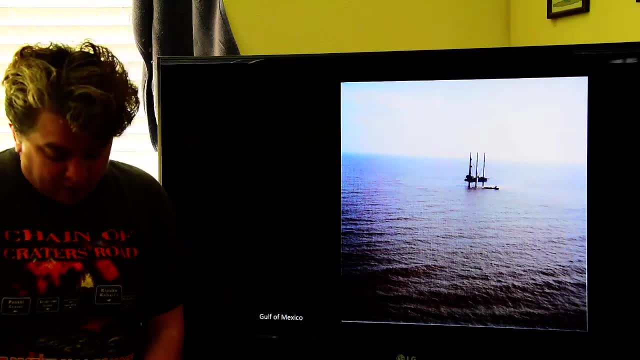 it sound like it's exactly like the 1800s, because it's not, Even though the basic principle is the same as that of the 1870s. That's how we drill the well And that's how we make it sound like it's. 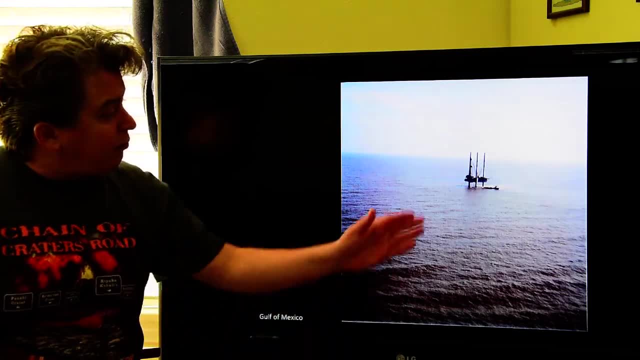 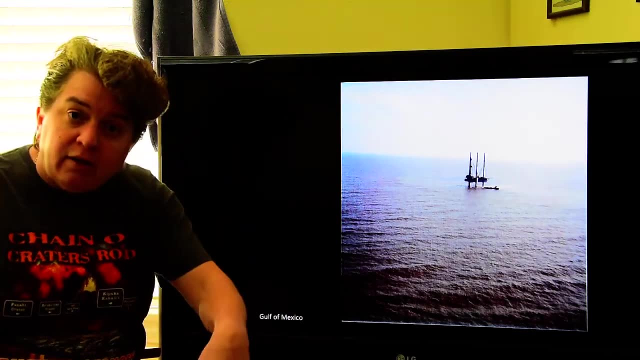 exactly like the 1800s, because it's not, Even though the basic principle is the same as the same of drilling into the rock. Nowadays we have offshore oil rigs. We can do directional drilling. We don't have to go straight down anymore. We can actually bend the drill stem to find the best. 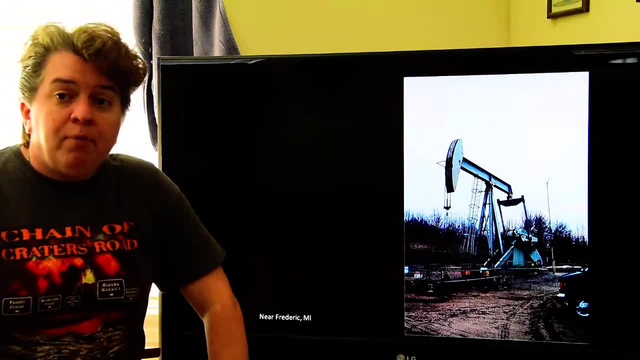 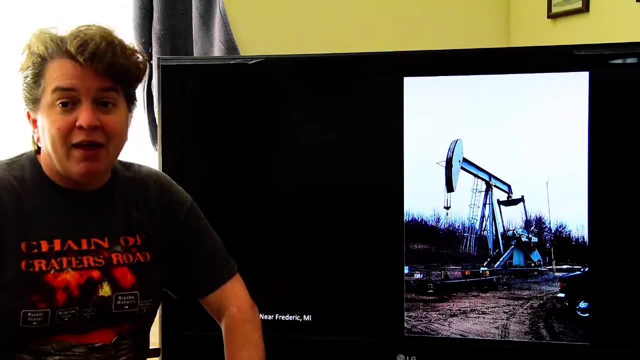 place to get to the oil. But eventually, once we've drilled that hole, we'll put a pump on like this: This is going to rock back and forth and it's going to pull all the oil out of there. So there you go. There's a little bit about the history of the oil industry. 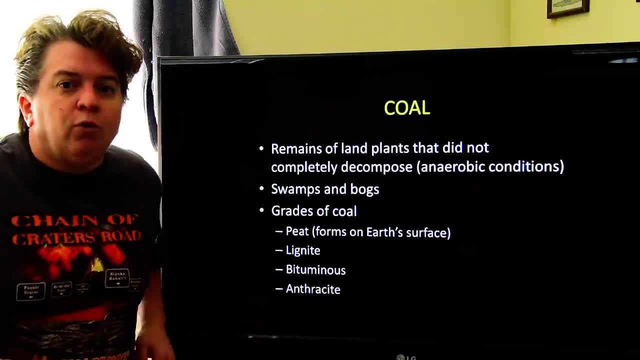 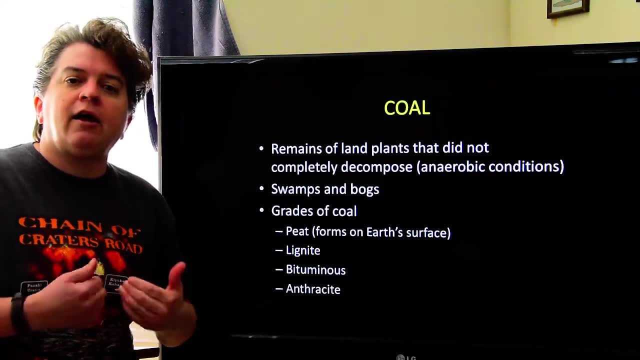 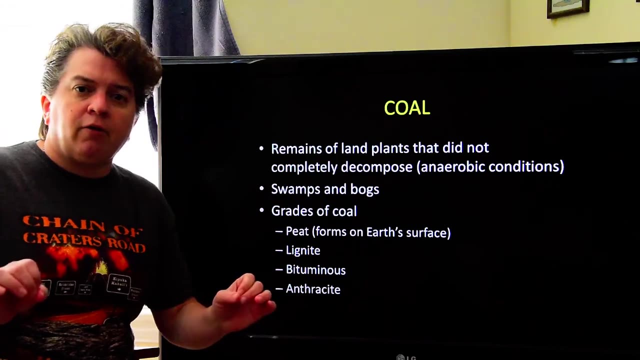 So let's move on to a different fossil fuel. This one's going to be coal. Coal, like I said, is also a fossil fuel, but the organic material that makes it comes from a different place than oil. Oil was marine microorganisms, right, The plankton that's off in the oceans. 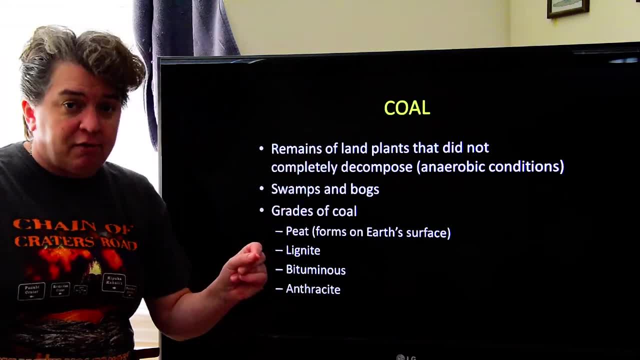 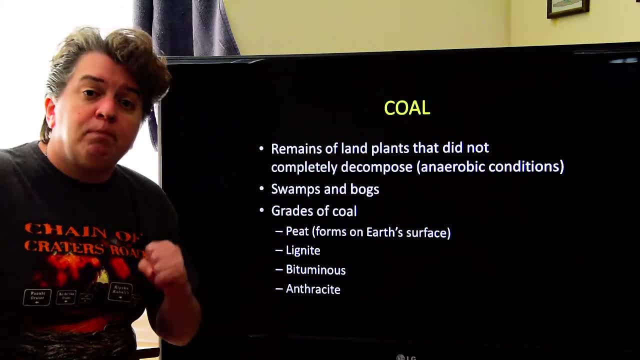 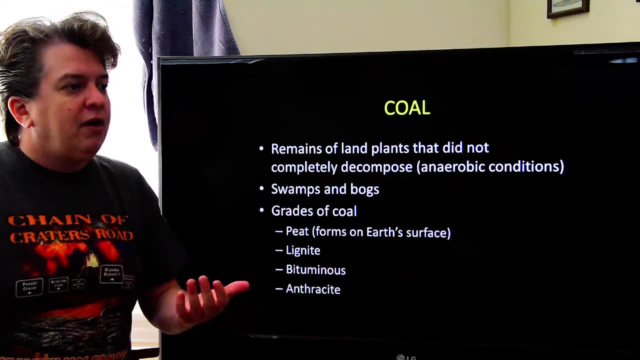 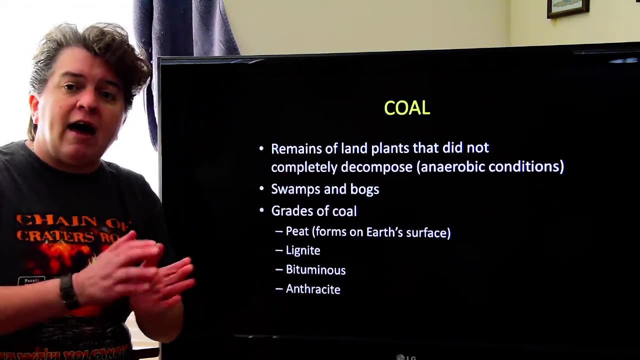 decompose So this organic material could build up over time. And what do we need for the material not to completely decompose? We need anaerobic conditions, low oxygen or no oxygen conditions That limits decay, And the environment where we tend to get that are in swamps and bogs. 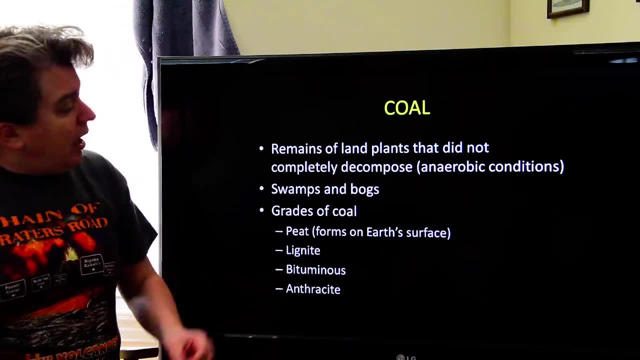 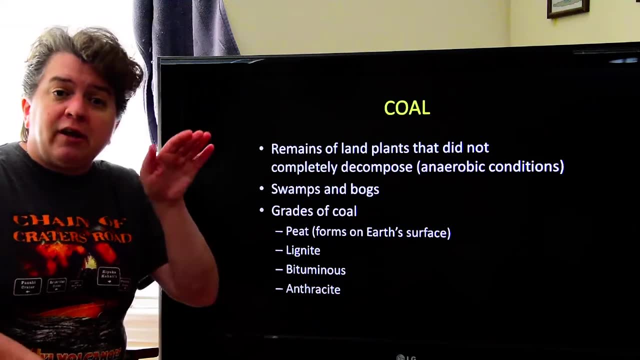 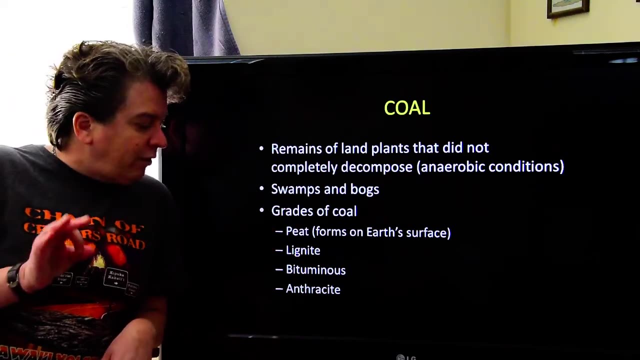 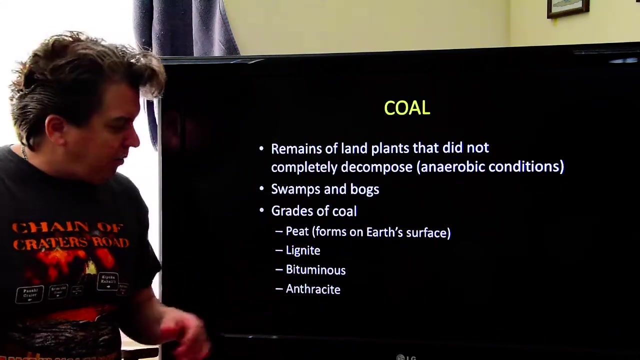 where we get stagnant water, And in these areas of stagnant water you tend to get this plant material to accumulate and eventually it can get compacted into coal. In coal we have different grades of coal that exist, And grades simply means kind of like how good they are And so low grade. 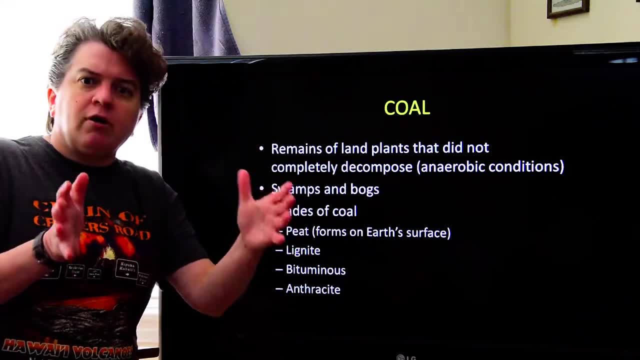 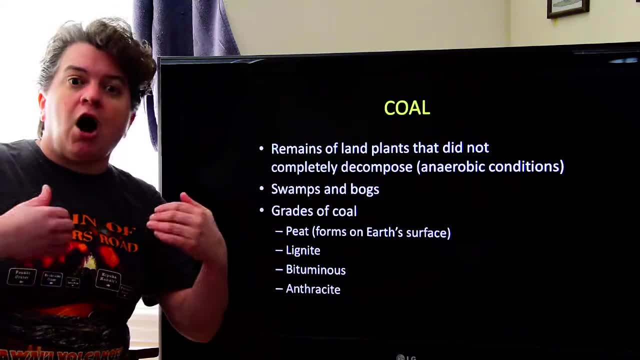 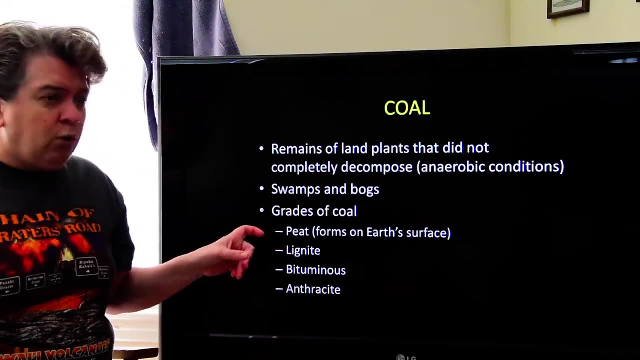 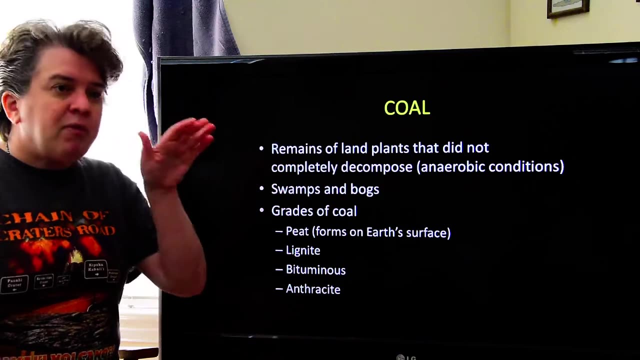 some high grade coal, same volume of that. it's going to produce a lot of energy and less waste. So that's the difference between low and high. So the lowest grade of coal, which is actually kind of pre-coal, is peat which you can find formed on Earth's surface. But then, as that peat, 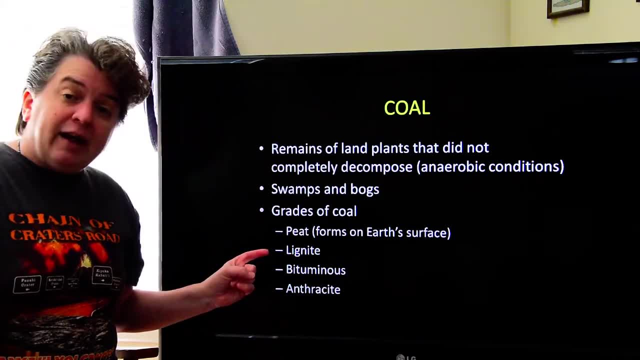 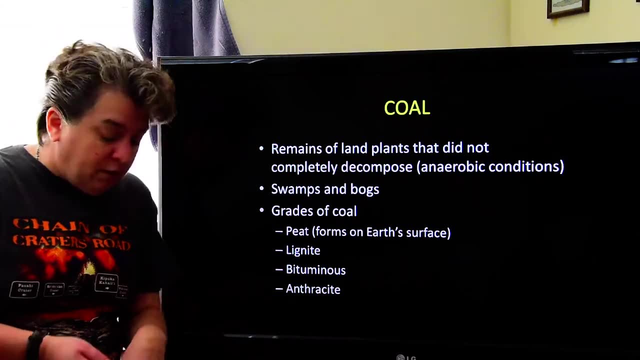 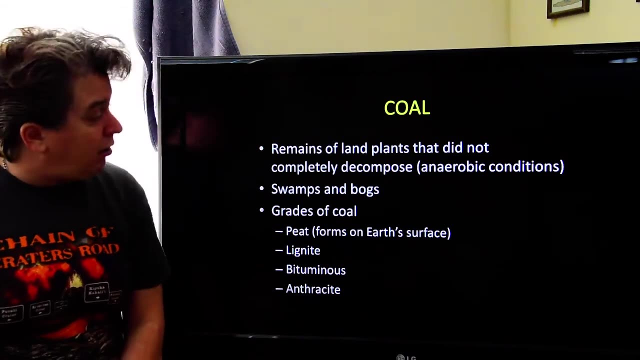 gets buried and compacted a little bit, it turns into lignite- Lignite, which is also known as brown coal. that gets compacted a little more and we get bituminous, And then the highest grade of coal is anthracite. It is also the rarest grade of coal, So that's. 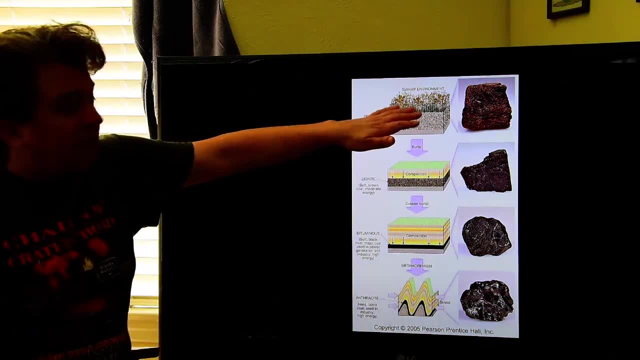 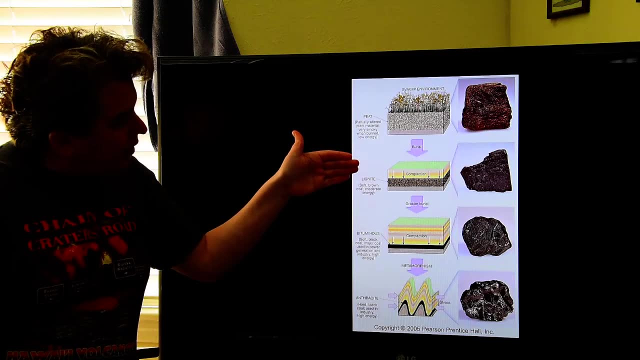 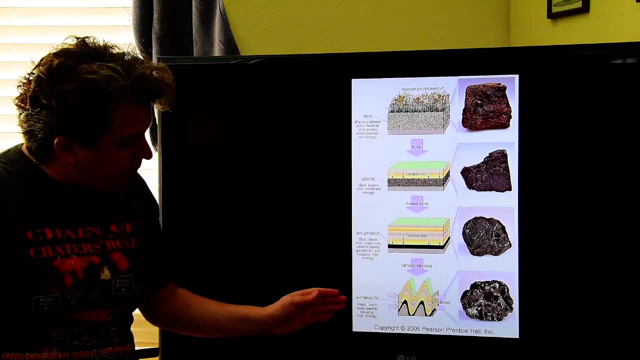 what we're looking at here. This is our peat that's developing in this swamp environment And it says, you know, very smoky when burned. low energy gets compacted into lignite, into bituminous coal And ultimately into this anthracite, if possible. And that gives you this description: hard black. 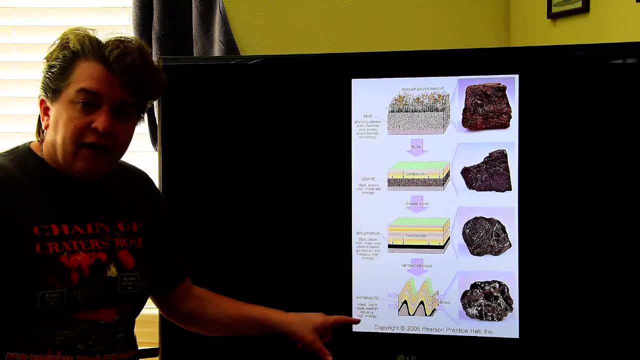 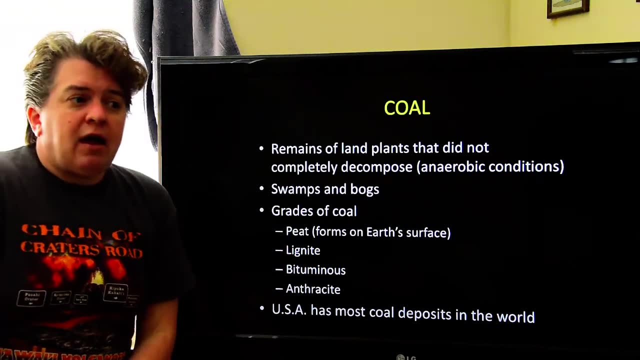 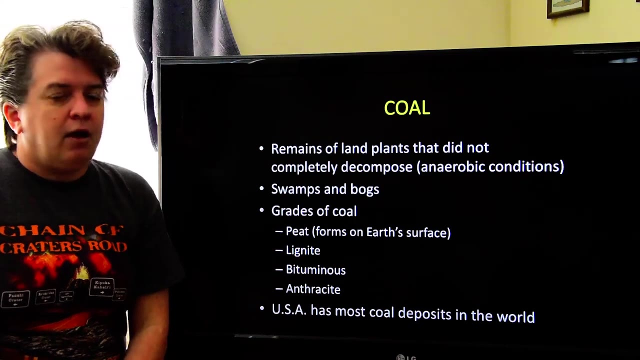 coal used in industry. high energy releases a lot of energy when you burn that, All right. The US has the most coal, the most abundant coal in the world, And I'm just watching my cats getting into trouble. The US has most coal deposits in. 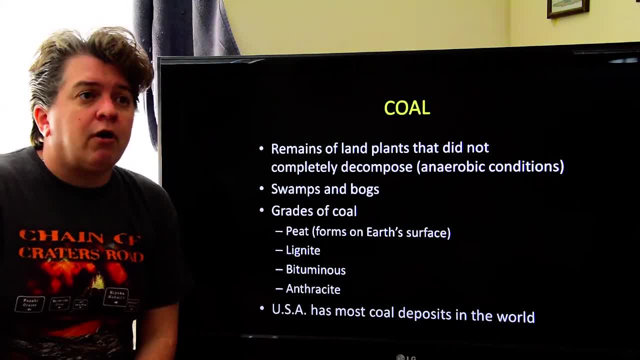 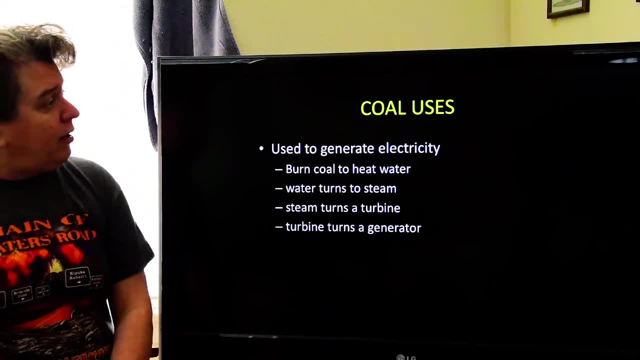 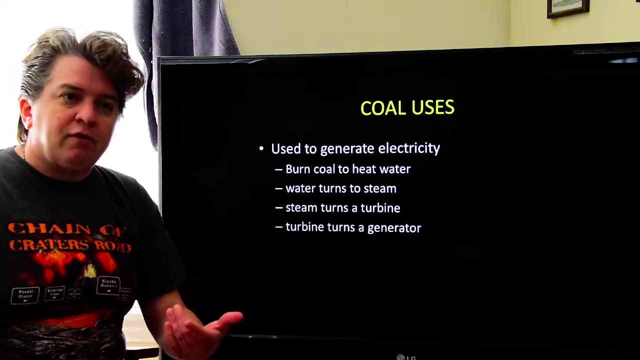 the world. But of course, these days, most countries are trying to get away from using as much coal, which we will talk about in a little bit. Now, what's the main use of coal? It's used to generate electricity, And this works like. 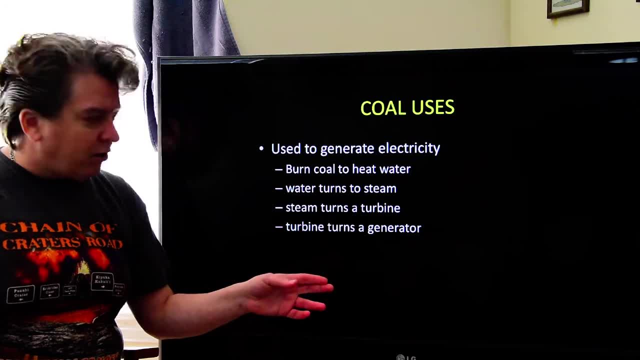 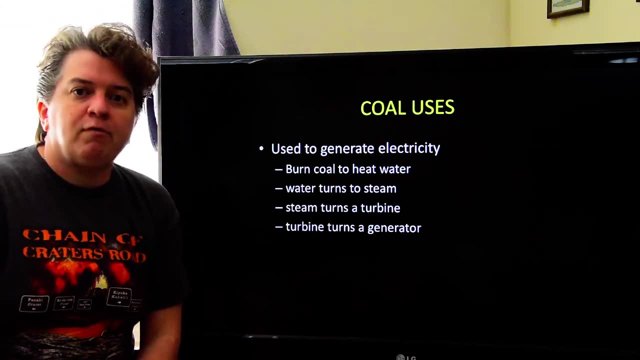 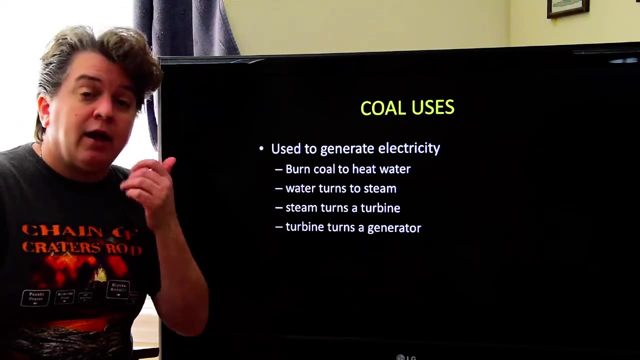 most other power plants, You burn the coal to heat water. The water turns to steam, The steam turns a turbine, The turbine turns a generator And this is how coal has been, or how energy has been generated. So electricity has been generated for over 100 years burning coal. And yes, we do still. 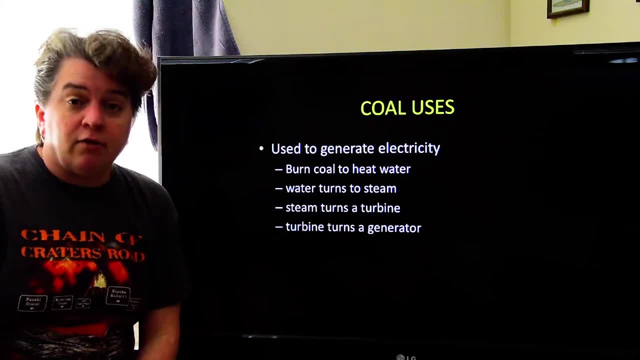 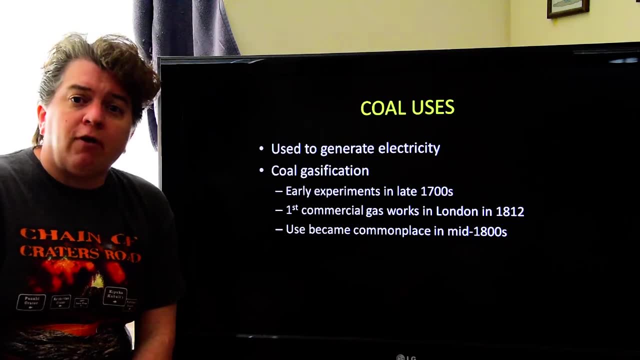 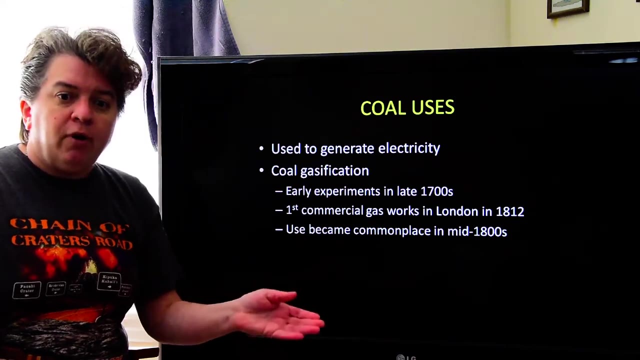 burn quite a bit of coal in the United States today to create energy, But coal can be used for other things. It's actually very versatile And it can be gasified. So you can take coal and through a complex set of processes you can actually turn the 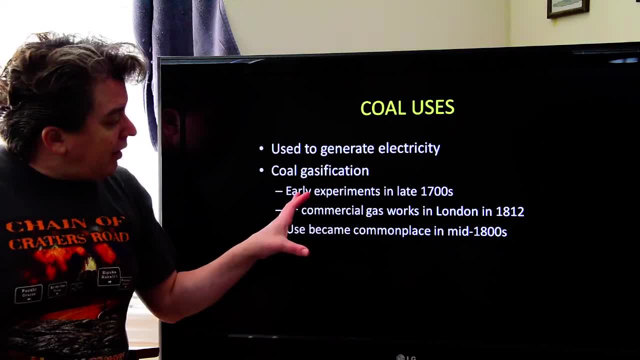 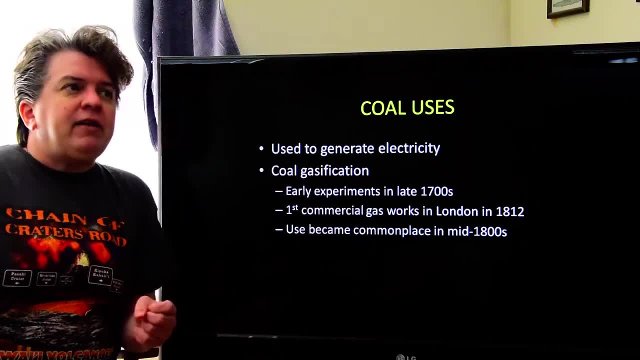 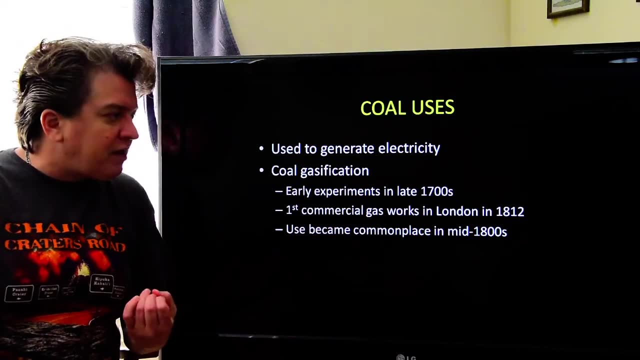 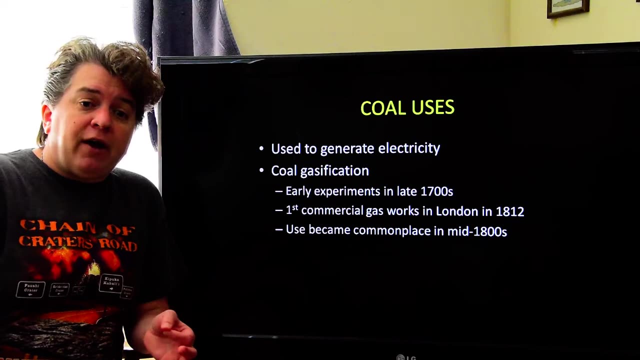 in the 1700s And finally really became economic by 1812. And we have this first commercial gasworks in 1812.. And then by the mid-1800s the use of gasified coal became very, very. 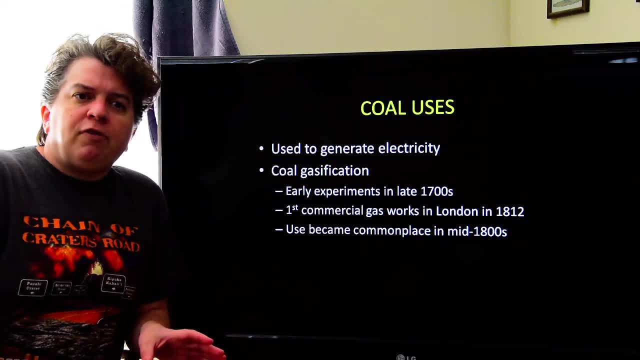 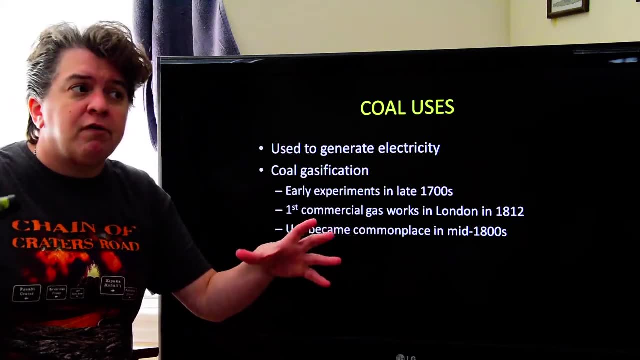 common. In fact, any city with a decent population quickly teach everybody that coal, coal, each song should be cut down- would have had a gas works and that gas would have been piped around the city, even to individual residences and instead of, you know, turning on the, the. 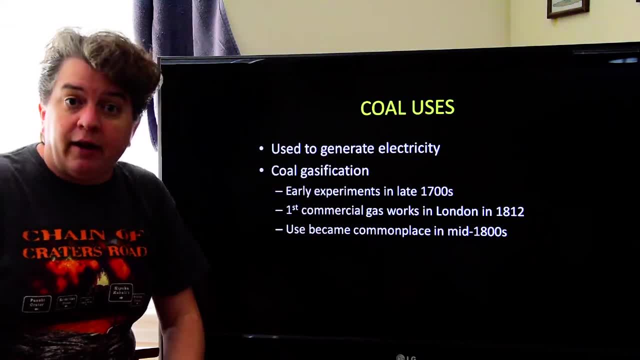 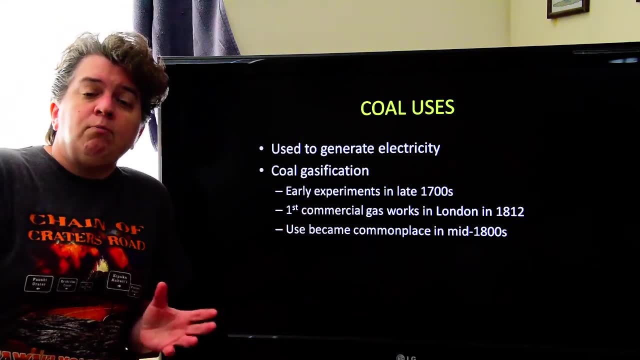 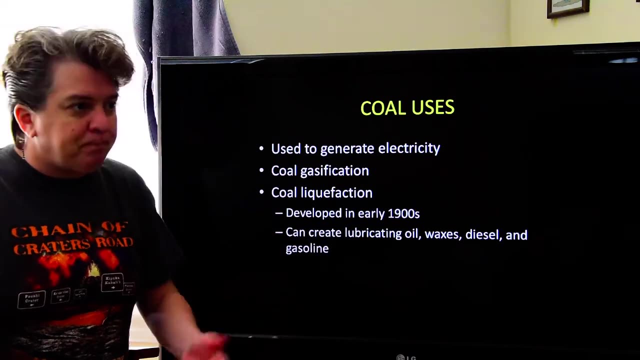 electrical lights. today you turn on the gas and light, light your gas lamp, and so gasification has been done quite a bit. we don't really do it much anymore because natural gas is simply cheaper. so why bother doing this when you natural gas is cheap? you can also liquefy coal. let coal liquefaction was developed in. 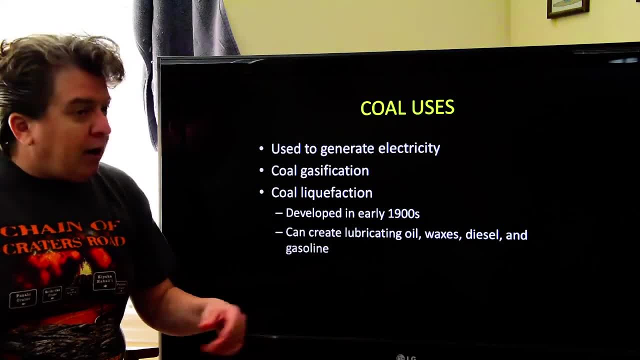 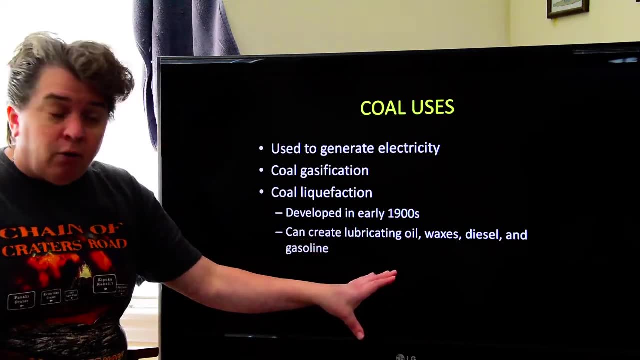 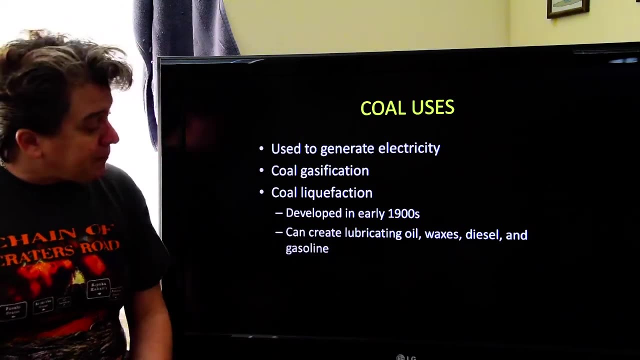 the early 1900s and basically what you can do. through again a bunch of complex chemical processes. you can create lubricating oils, waxes, diesel fuel and gasoline from coal, and this is again we don't really do it much, but you can do it if you want to do it. if you want to do it, if you want to. 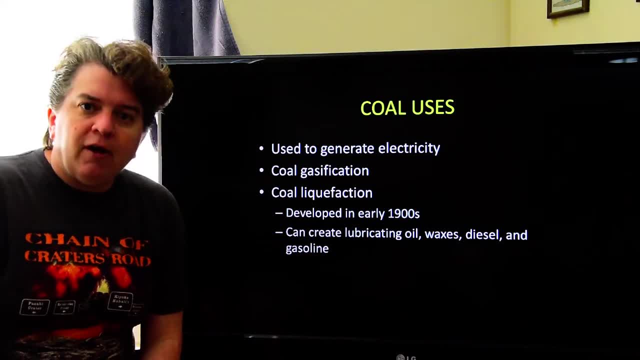 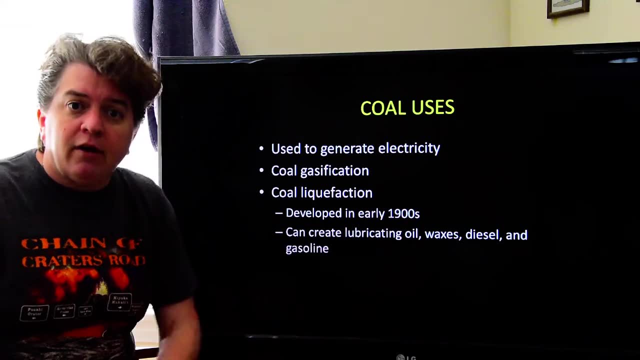 do it much today because it's expensive. right, it's a lot cheaper to get some oil out of the ground and refine it and turn it into diesel fuel and gasoline and these other things, but it's not that we don't have the technology to use the. 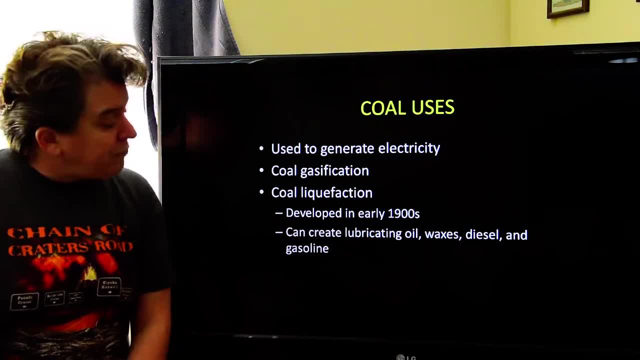 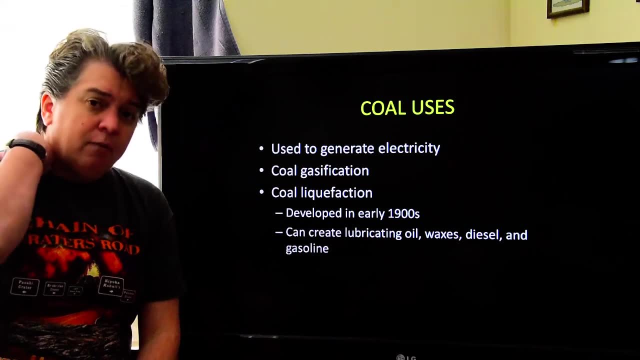 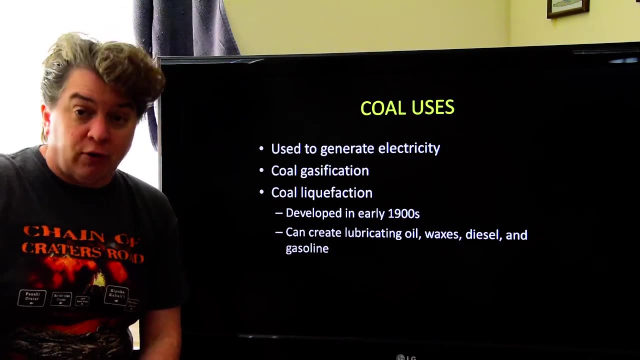 coal in that way in the Second World War, and Germany actually used a lot of coal liquefaction, because Germany does not have a lot of oil deposits, but they do have a lot of coal, and so of course many countries weren't going to be trade trading with Germany, because they 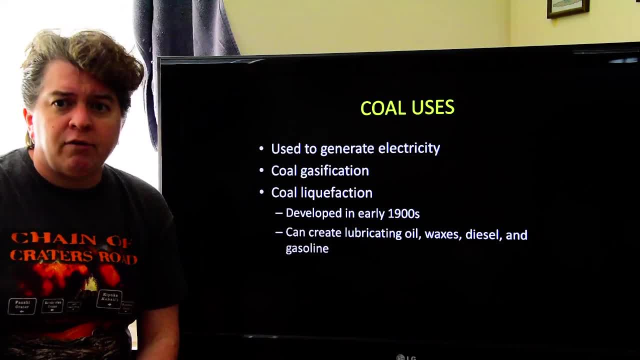 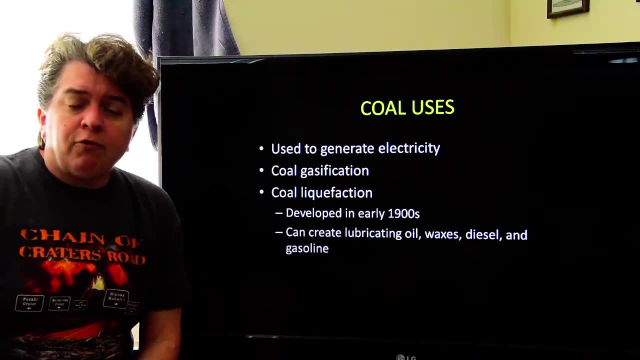 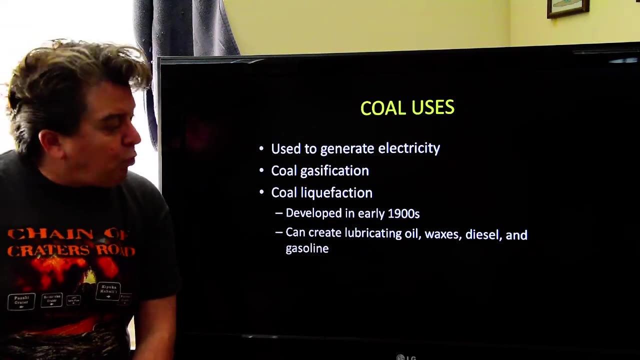 were a bunch of like absolutely creepy, crazy, whack-job Nazis, and so they had to, you know, make their own energy, and so a lot of liquefaction of coal was done during the Second World War for Germany to power, you know, their airplanes and tanks and things like that. more recently, South Africa, when they were still under. 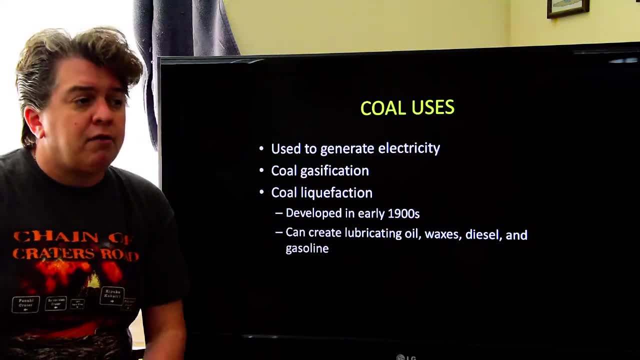 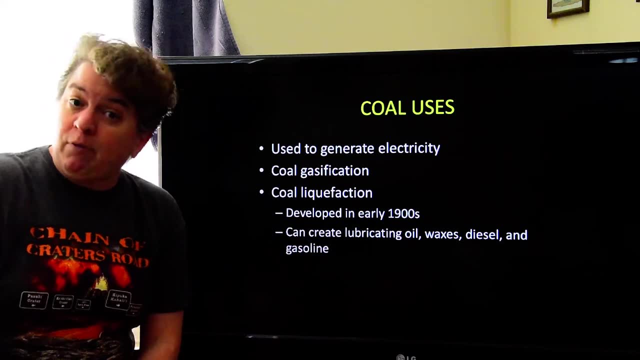 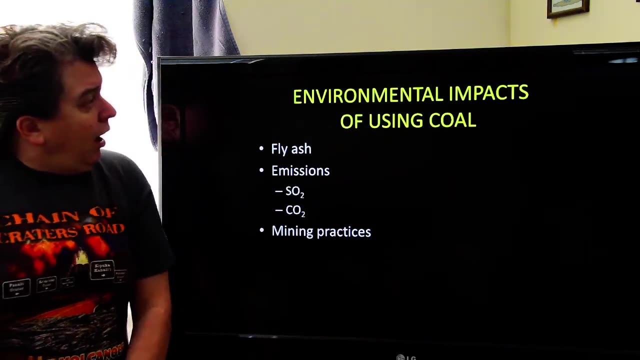 apartheid rule had to liquefy coal. because, again, they had to liquefy coal and apartheid was terrible and no one wanted to trade with them, and so they had to use a domestic source, which happened to be coal, and so it was liquefied as an energy resource. all right, now coal is cheap to use to. 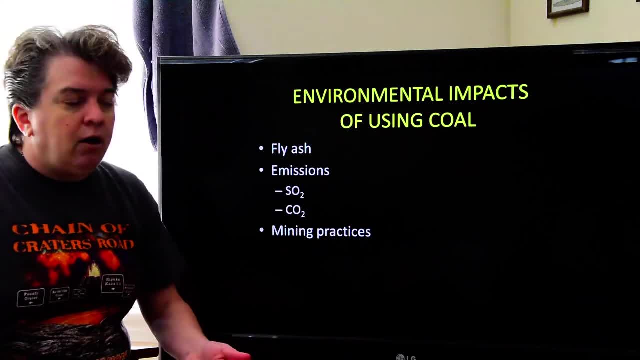 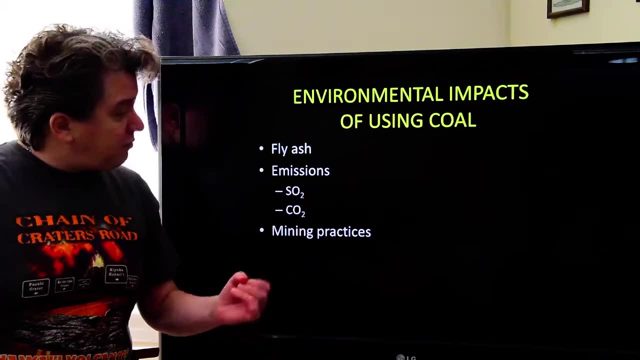 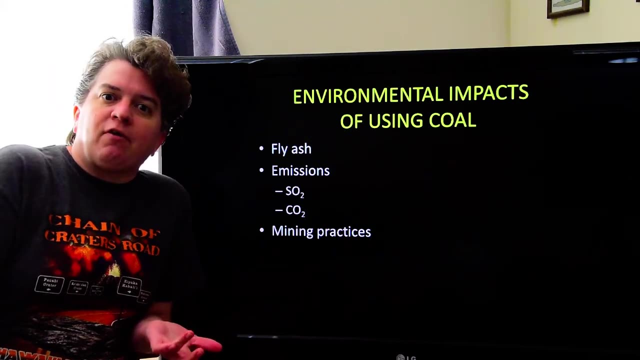 generate electricity. it's versatile. however, there are drawbacks to using coal. when you burn coal, you get waste and we call this stuff fly ash, and I mean everyone should kind of understand this. if you've ever had a campfire right, there's ash left over in the morning, while burning coals the same. 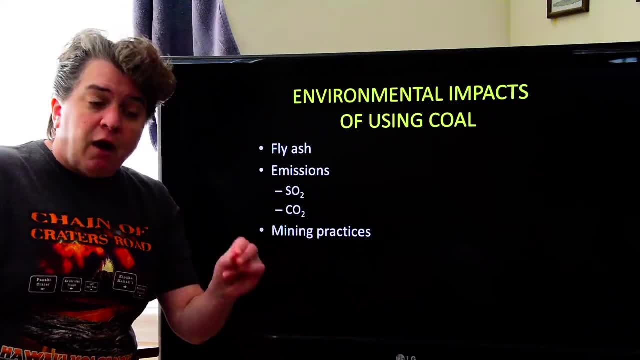 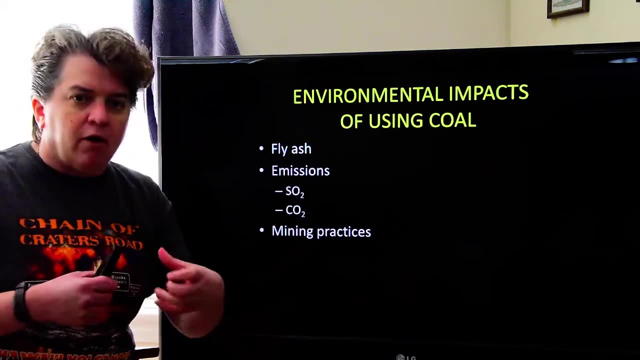 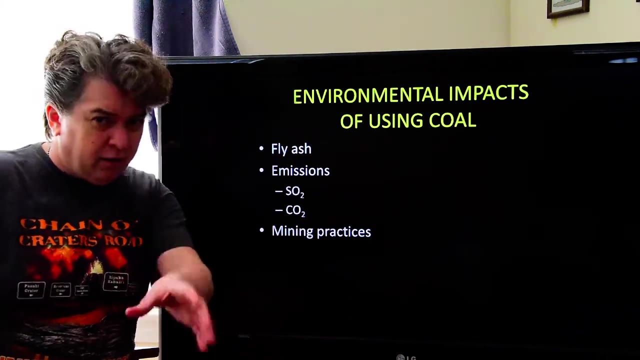 way, this fly ash. some of it is used in making concrete. you add a certain amount of fly ash to concrete and it gives the concrete different characteristics, like better tensile and compressional strength and stuff. I don't know exactly what it does. I just know that it's used in concrete making, but not all the fly. 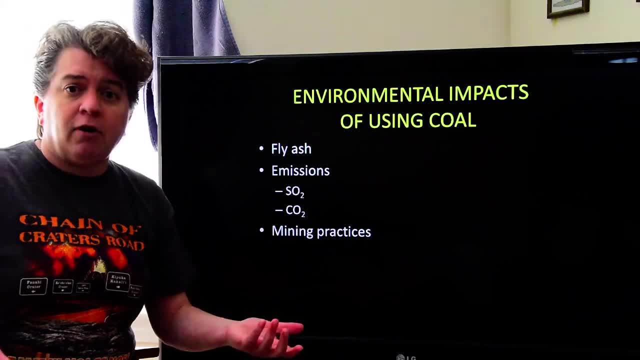 ash generally is used in making concrete, but not all the fly ash generally is used in making concrete, but not all the fly ash generally is used in making concrete. so we have this stuff left over and we have to think about where are we going to dispose of it. then there's, of course, 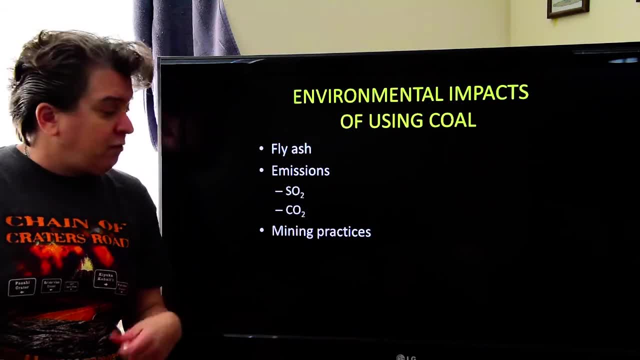 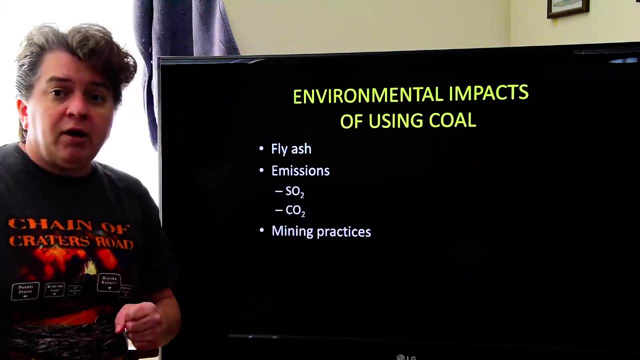 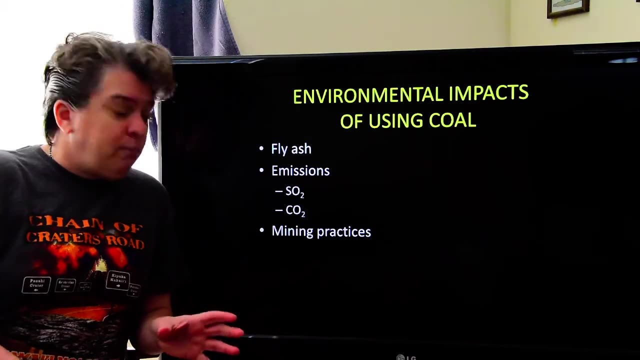 also the emissions that can be produced from this. sulfur dioxide can be produced, which can cause acid rain. we have carbon dioxide, which is a greenhouse gas. you can also have mercury released, and so there are considerations about the emissions from that. and then, of course, there are the mining. 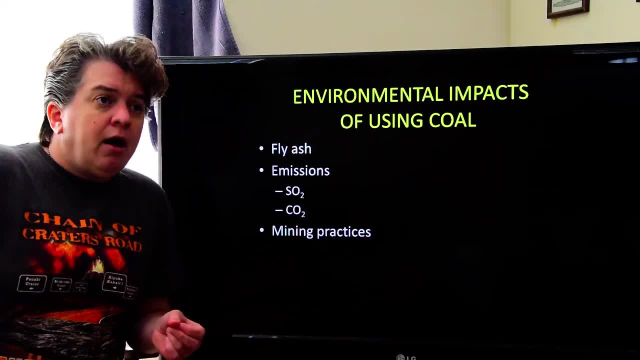 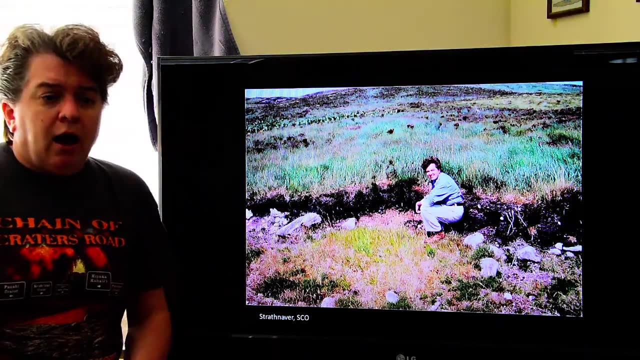 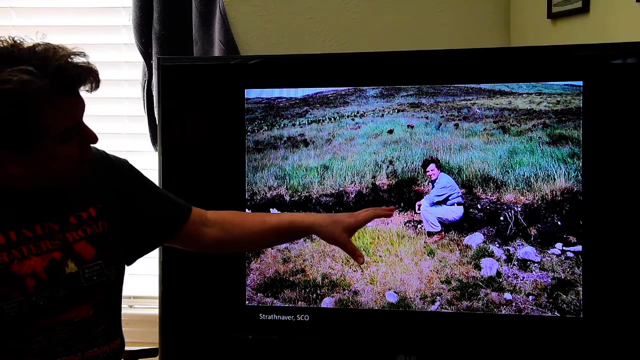 practices. coal mining is really the most dangerous sort of mining that you can do, and we're going to talk a little bit more about that in a little bit, but I just want to show you a few things about coal. so this is peat forming off in the 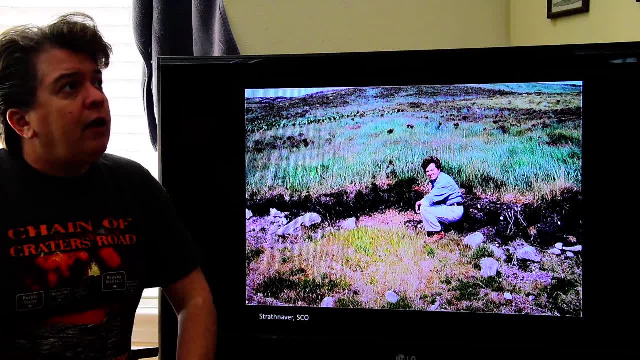 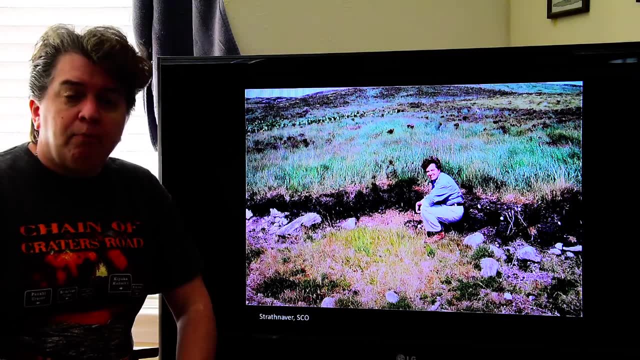 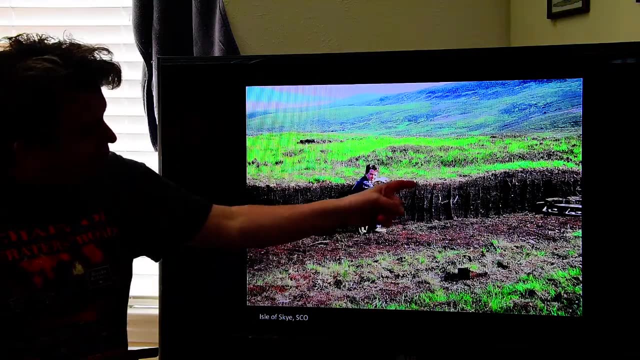 Highlands of Scotland, and in the Highlands and also in parts of Ireland and parts of Scandinavia, they still cut peat and burn it like you might burn logs in a fireplace in winter time, and that's what we're looking at right here. here's where some of this peat has been cut out of the ground. it gets stacked to dry out. 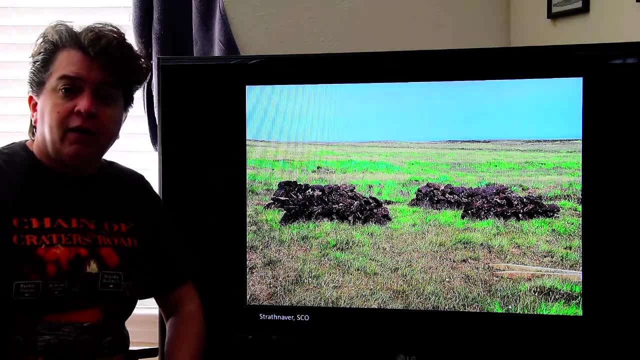 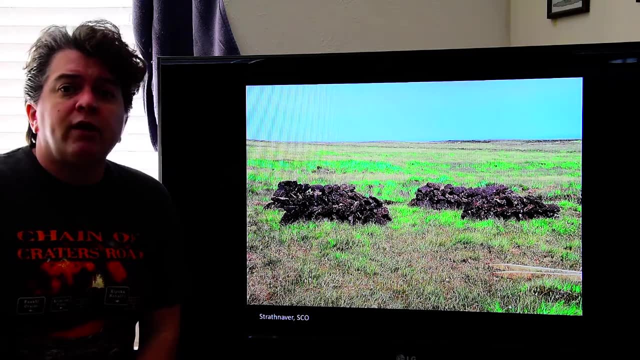 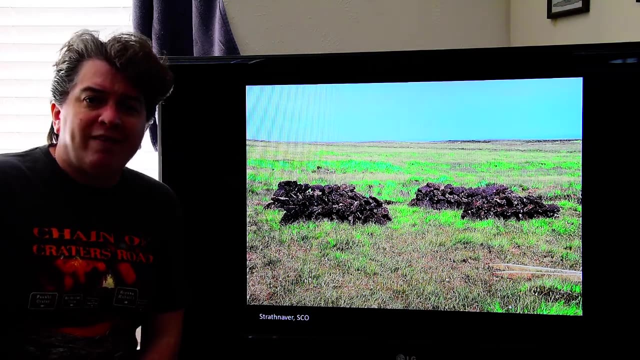 and then in winter, instead of, you know, throwing another log on the fire to heat the the house, you know, just go out and get one of these bricks of peat and put it on the fire. it produces a really smoky fire with a distinctive smell to it and, if you like, scotch whiskey. 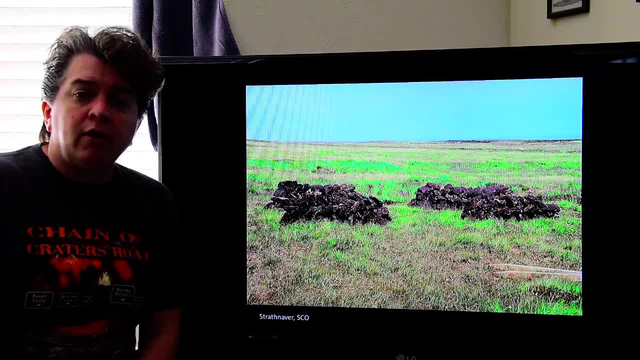 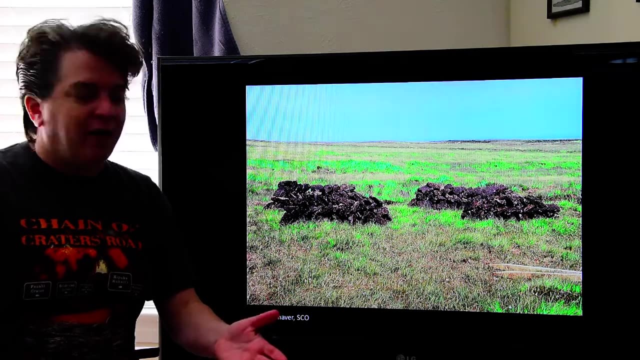 you like peat, because an important part of making scotch whiskey is the molting process, where your barley is basically smoked in a peat fire, and so that's part of what gives scotch its name and that's why it's called peat fire. 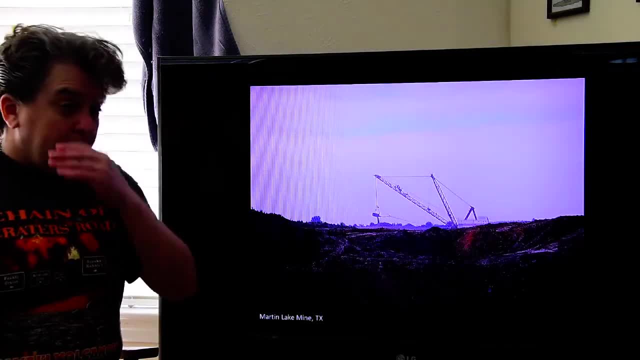 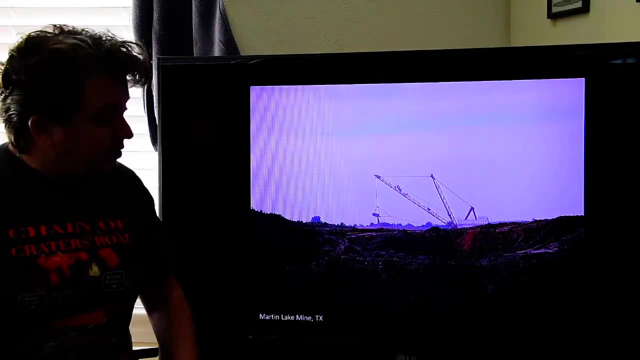 I'm just going to show you a little bit more of the difference between the two of them. now, distinctive flavor. okay, how do we mine for coal? you might mine for it using a strip mine like this one. we talked about strip mining in a previous lecture, where 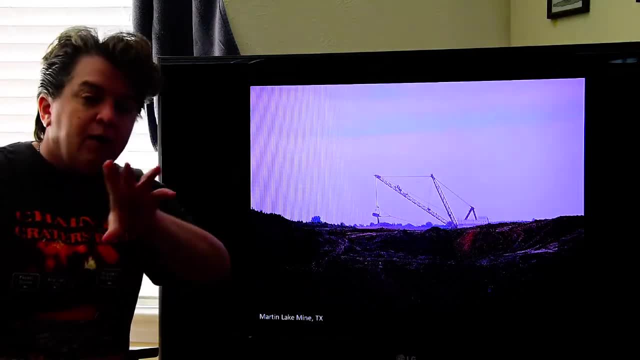 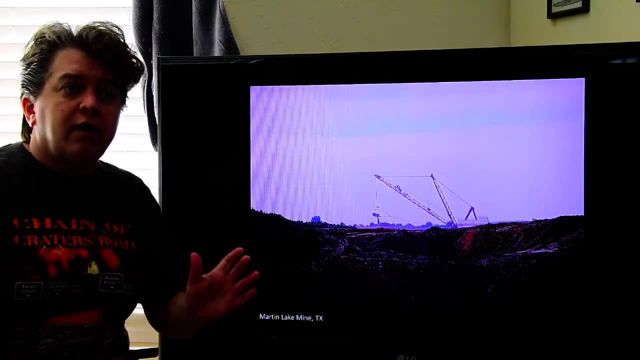 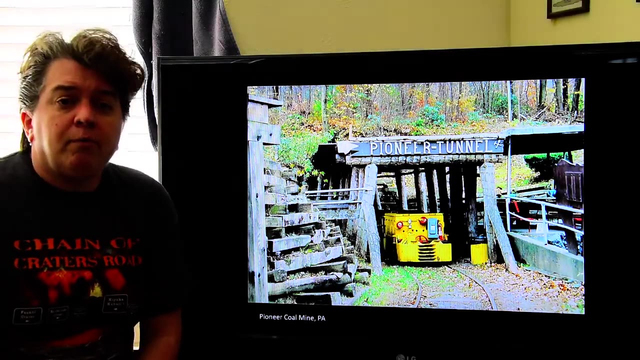 you basically scrape the material off and then put the soil back in place and reclaim the land. that's what we're seeing here at the Martin Lake mine. this is in Texas. if you drive up US 59, you'll eventually run into it. coal can also be. 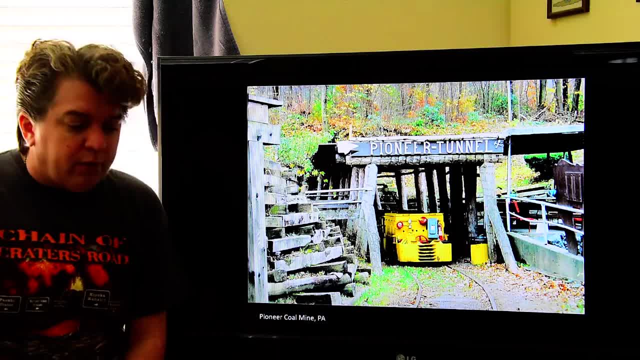 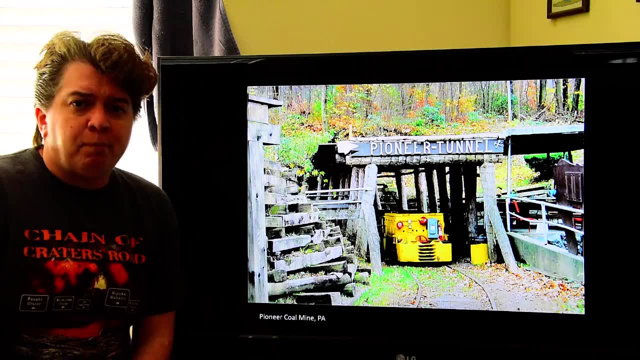 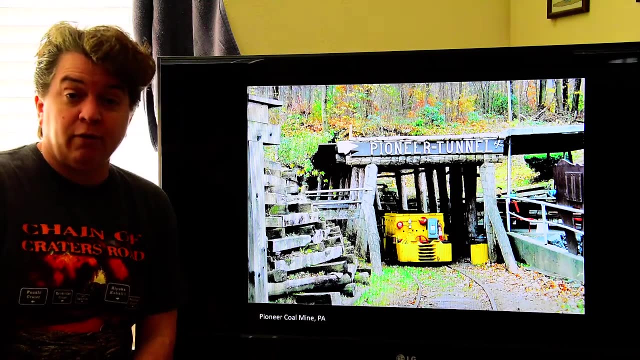 extracted underground and, like I said, coal mining is one of the most dangerous types of mining around. in fact, my dad, he, was an expert in coal mining and he told me don't ever work in a coal mine. he actually that was one of the only things he's ever asked me not to do is work in a coal mine. so I never have, but I have. 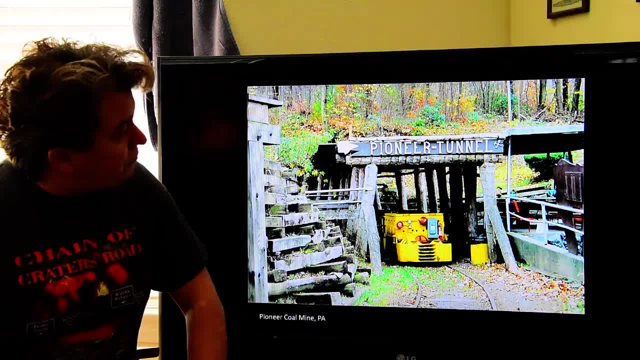 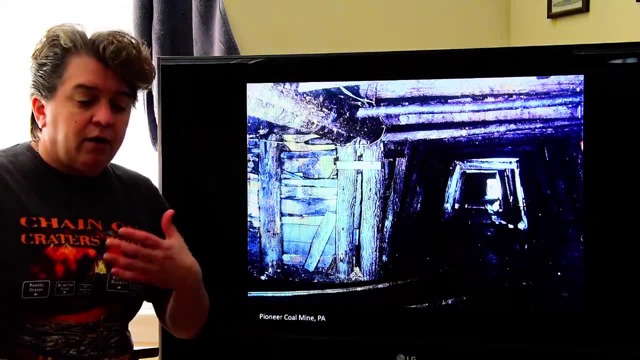 gone in a few coal mines. this is an underground coal mine and this is what it looks like underground. I know in the previous lecture I showed you what it looked like underground in a hard rock mine, basically in a copper mine where my husband used to work this. 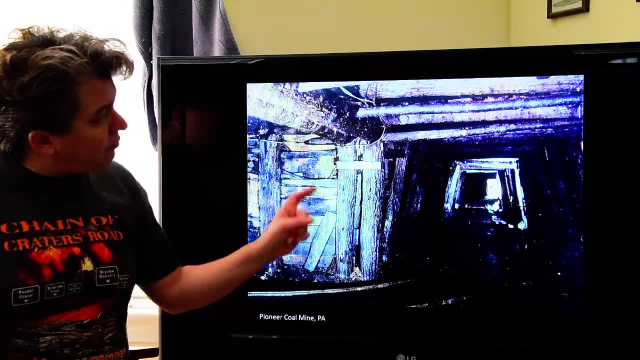 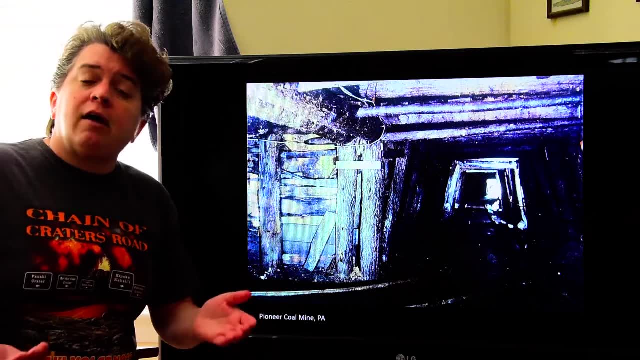 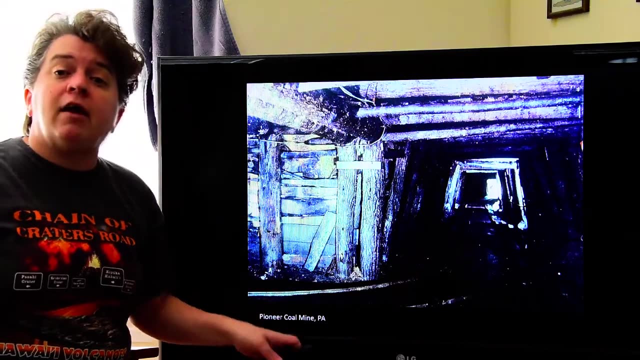 is going to look very different and, hopefully, why it looks different. you can see it has lots of timbering in it and you get all this timbering because coal is a sedimentary rock. sedimentary rocks form in layers. the layers are much more prone to collapsing than other rock types. 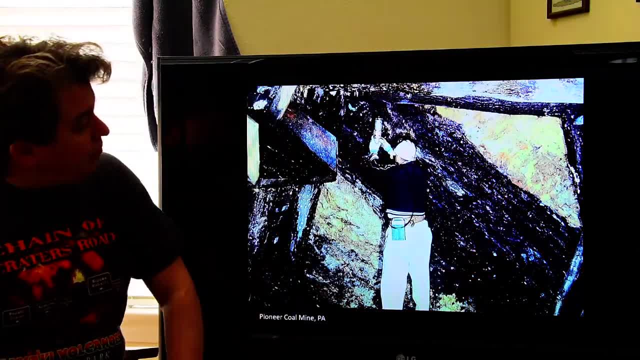 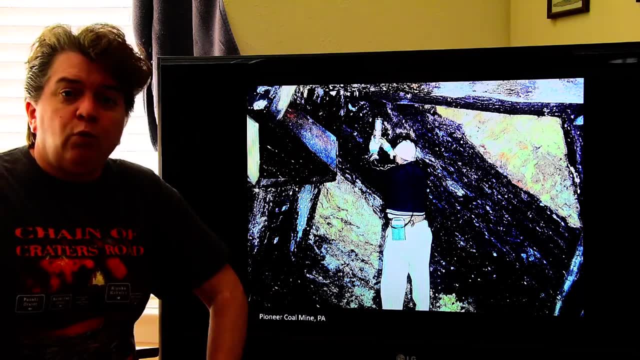 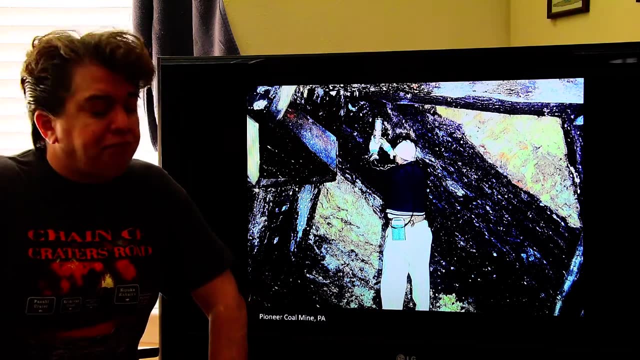 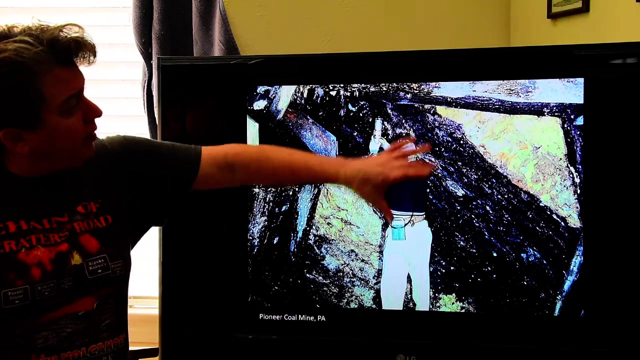 and you can see that here. this is a coal layer underground, and here's another reason why coal mining can be exceptionally dangerous. you can get some really weird gases accumulating in coal mines. you can get something that is called- what's it called? methane? methane is explosive and flammable and it can accumulate towards the top of the mine tunnel because 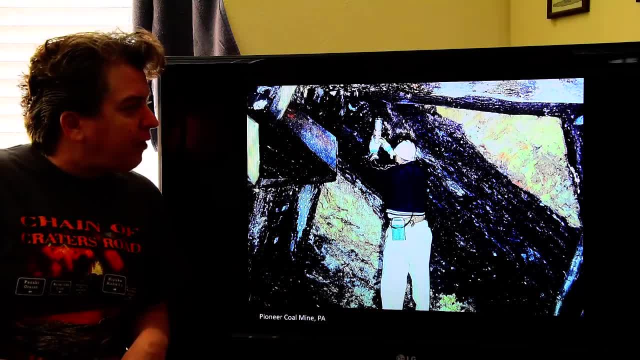 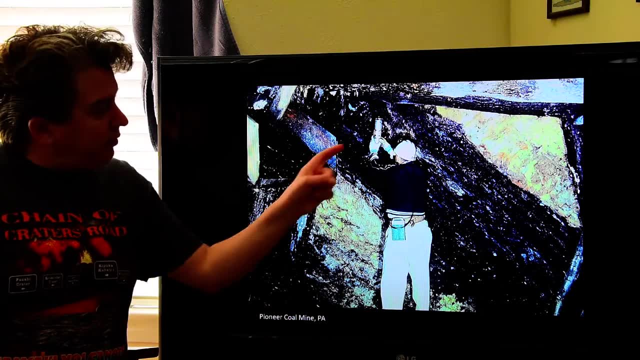 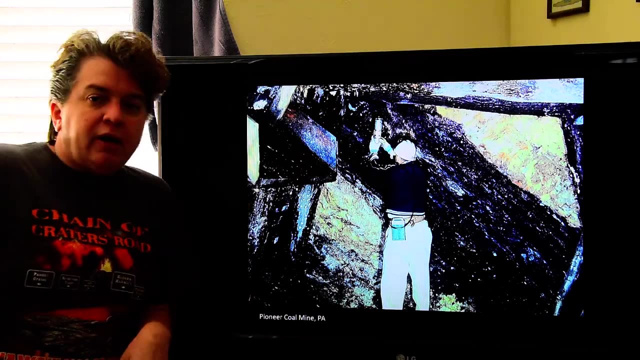 it's less dense than the normal atmosphere, and that's what this guy's actually checking for. he has a special type of lantern called a safety lantern, and there's a little flame in there that will get larger if- if there's methane present, there's other weird gases. 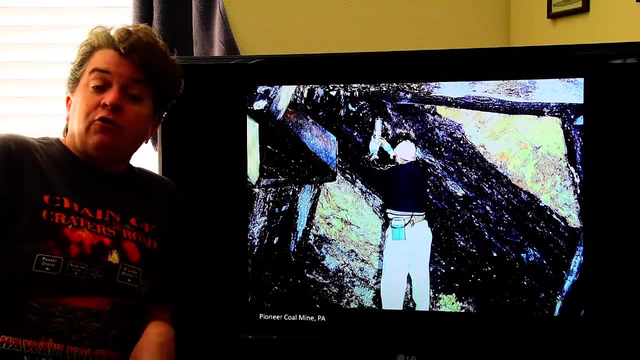 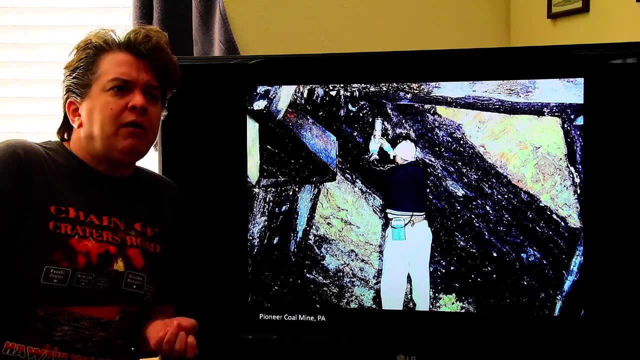 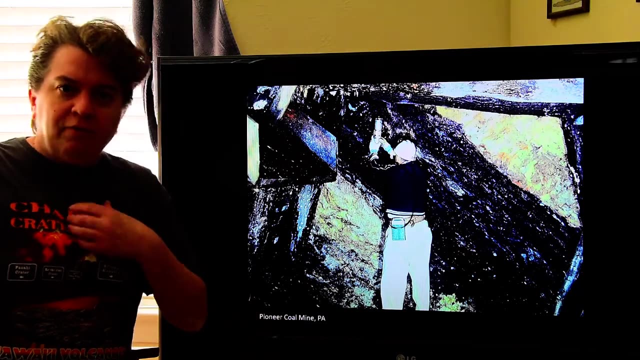 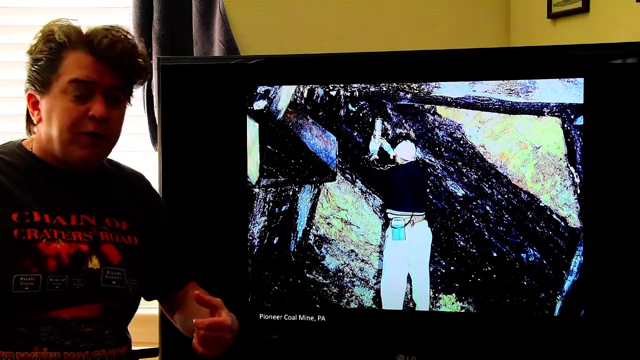 that can accumulate in coal mines that the miners have these interesting names for, like black damp and white damp, and they tend to be accumulations of carbon dioxide, carbon monoxide and nitrogen notice, no oxygen which we need to survive. they tend to accumulate towards the bottom of the mine tunnel because they are denser than the normal atmosphere. 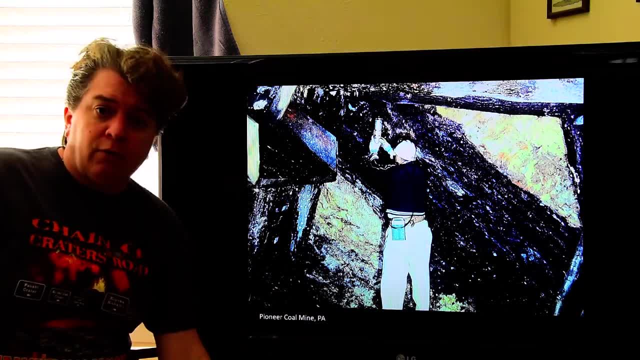 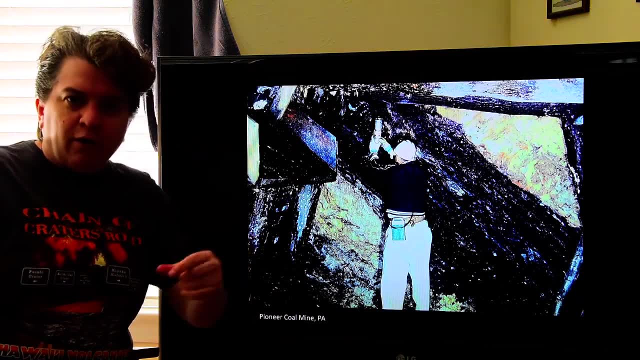 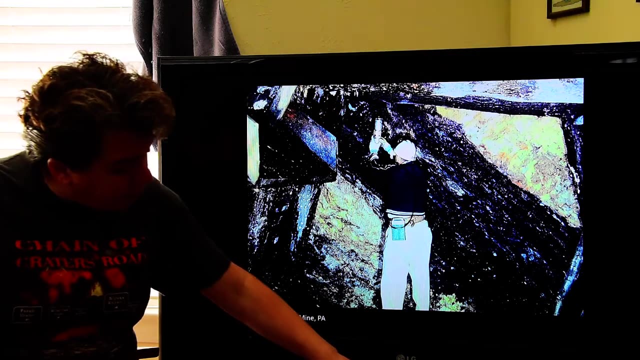 so you can take that safety lantern, hold it down towards the bottom, towards your feet, and remember the fire triangle. fire needs oxygen to live. if you see that flame getting smaller, you know to get out because there's this low oxygen mixture. in fact, if you go into mining engineering, there is an entire aspect of mining engineering. 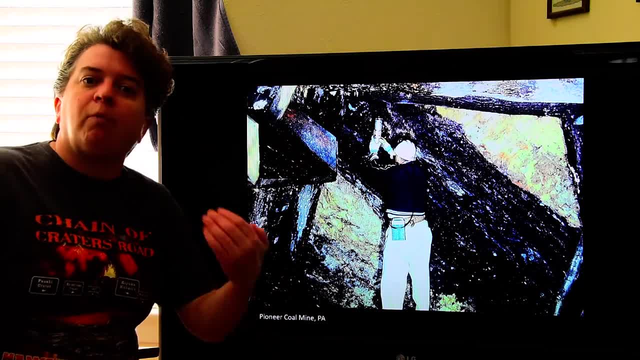 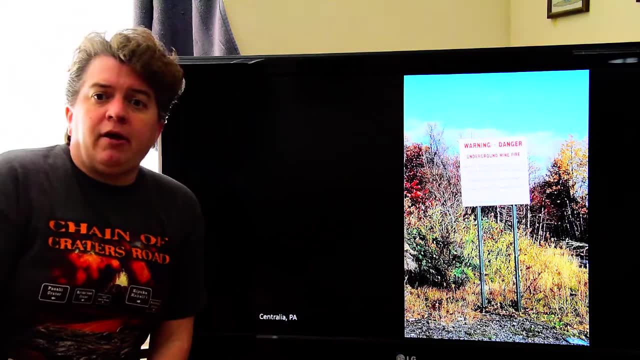 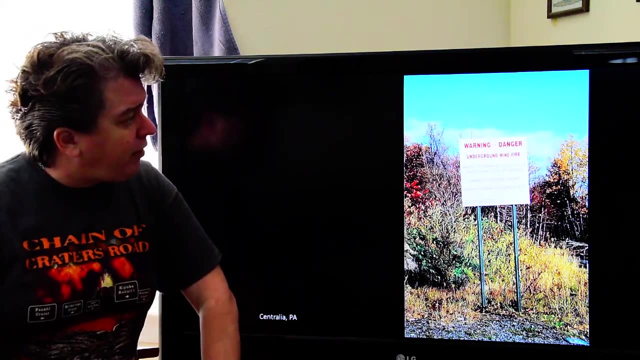 a specialty of making sure mines have proper ventilation so you don't get accumulations of these weird gases. coal mining can also be quite dangerous because it is flammable and we can see on this sign here it says: warning danger underground mine fire. walking or driving this area could result in serious injury or death. this is just a couple of miles away. 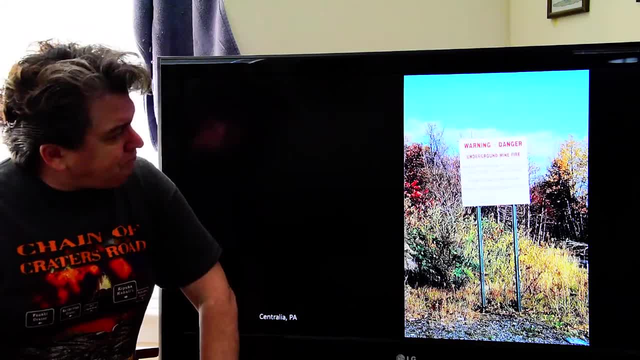 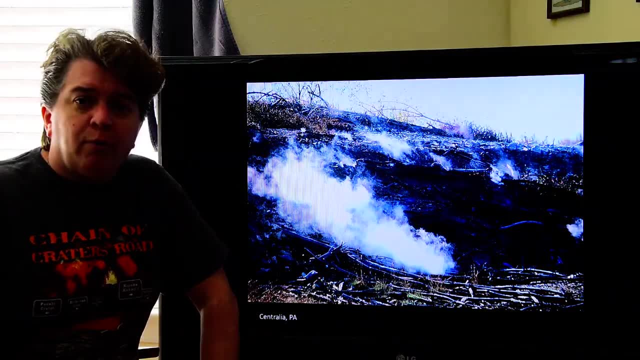 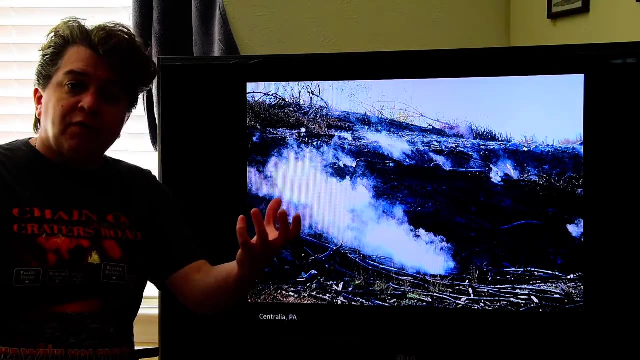 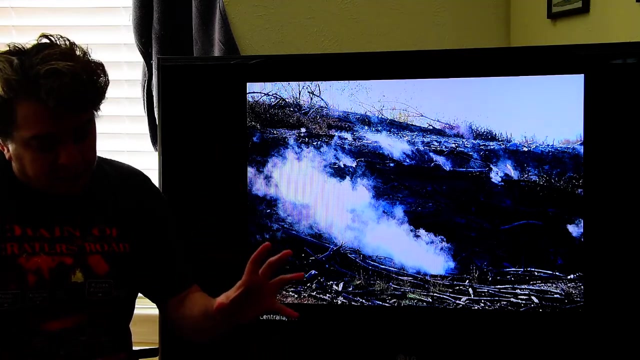 basically where I was born, And what happened back there was back in the 1960s in Centralia, Pennsylvania. people were burning garbage in an old mining pit and some coal was exposed at the surface there and the fire spread to the coal, and then the fire just started following the coal underground And so 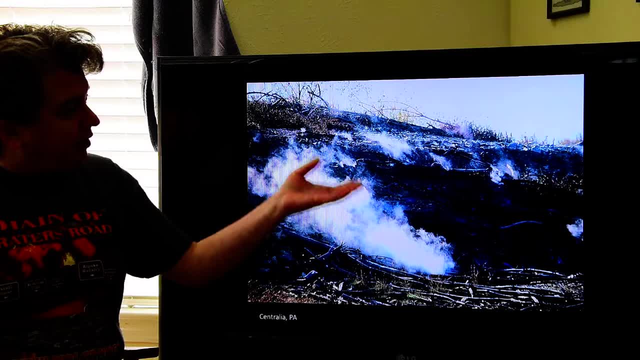 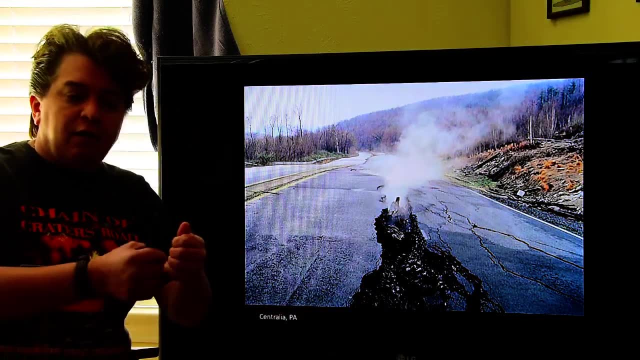 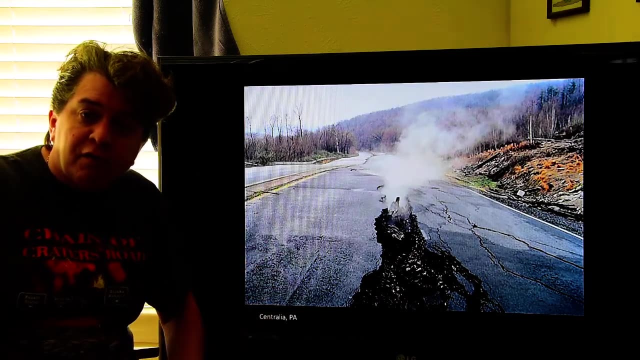 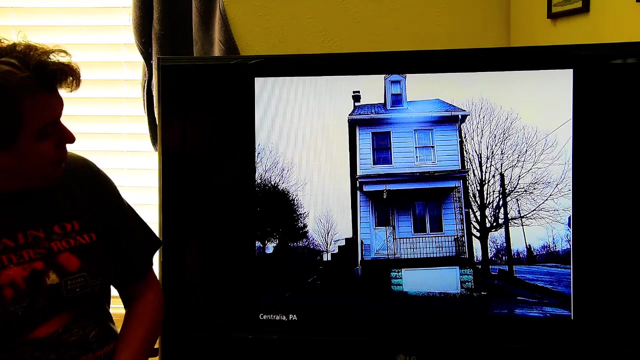 now, when you go around Centralia, you see all this land that's just steaming and smoking. It's very hot in areas. You get all these cracks developed because as the coal gets burned away it's smaller volumes, so the whole ground is shifting and settling in those places. Let's see. you see houses like this. So let me tell: 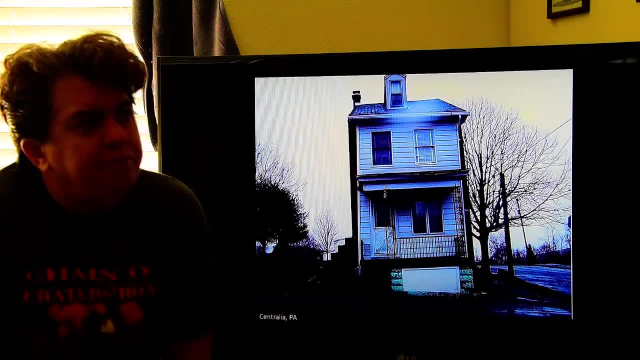 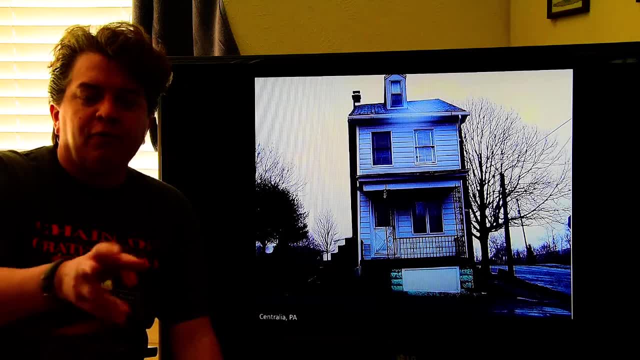 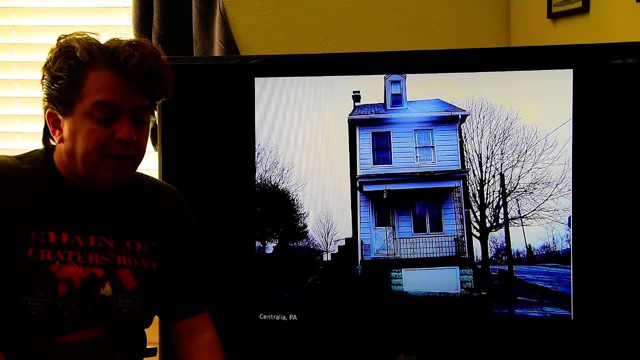 basically like fell into this fiery pit of doom. Fortunately his cousin was right with him and pulled him out before any serious injuries could happen. And after that happened, the government determined that they they wanted to buy out everybody who lived in Centralia because it was just too damn dangerous to live. 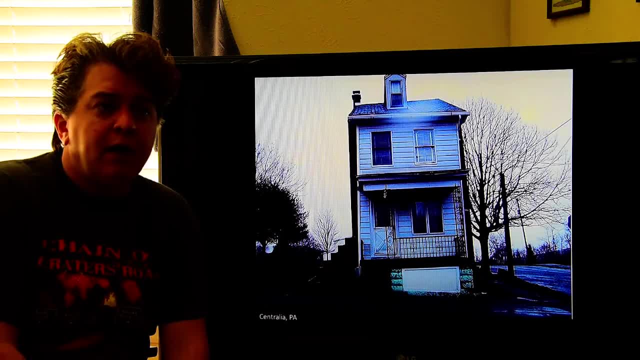 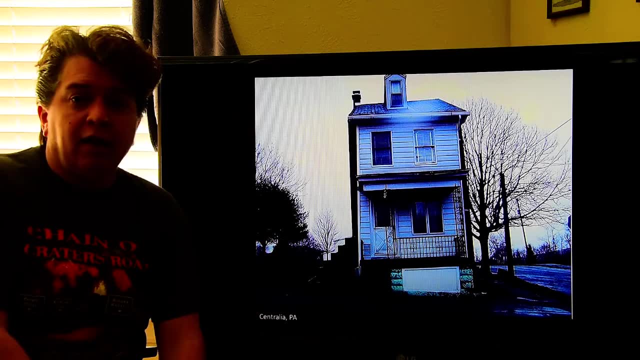 there, on top of this mining mine, fire. And so that's what happened: The town doesn't really exist anymore. There's only a few houses left of people who absolutely positively refused to leave the town, even though they were offered fair prices for their homes. But you might be asking: why didn't they just 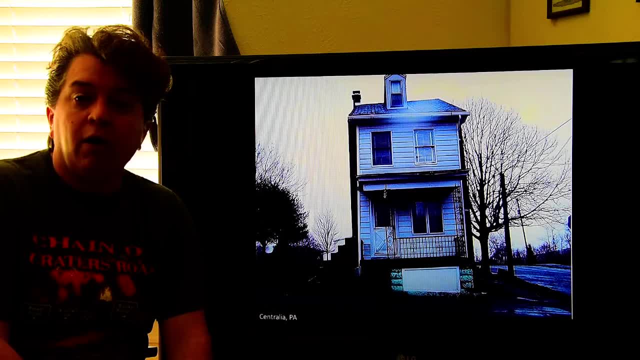 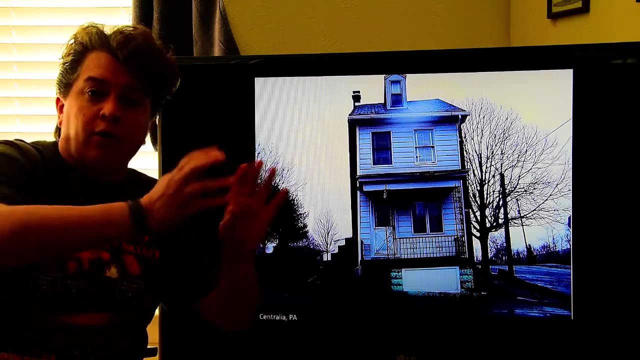 put out the fire? Why didn't they just like flood it with water or something? Well, mine fires are notoriously difficult to put out. In fact, the the only way you really can put them out mine fire is by digging it out, digging out the burning part of the coal, And that has been. 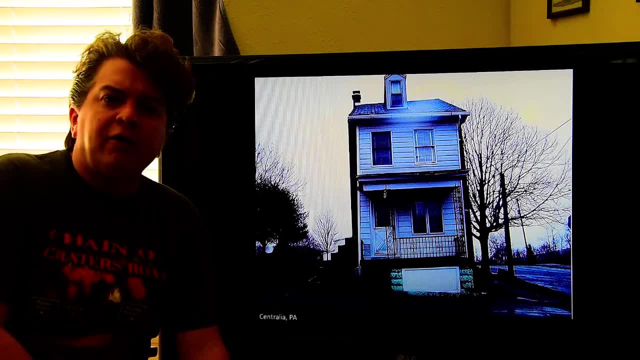 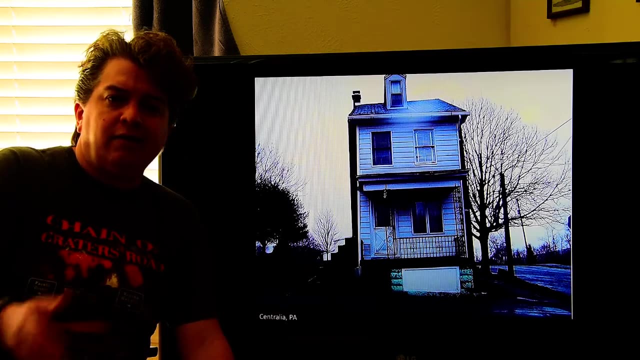 successful in some places around Minersville, Pennsylvania and I think, around Gordon Pennsylvania. they successfully did that a few times, This one unfortunately early on in the fire. if they wanted to dig out the mine fire they would have had to dig up the local cemetery. 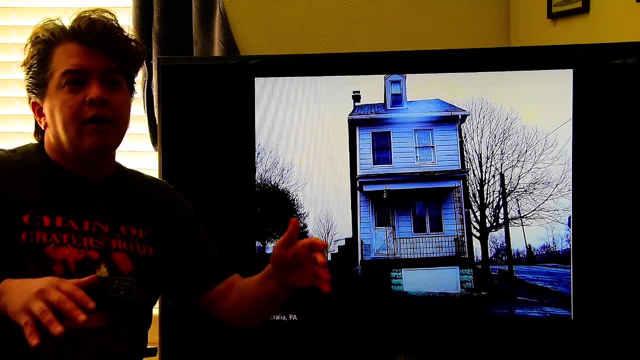 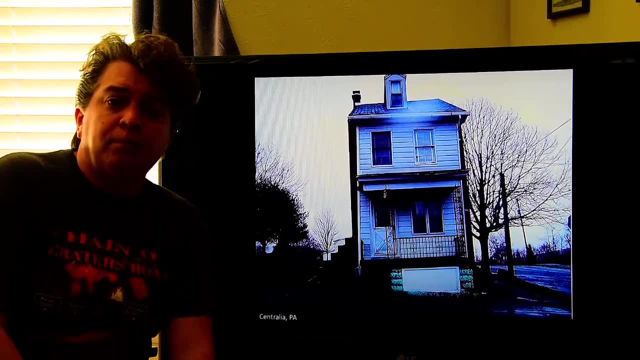 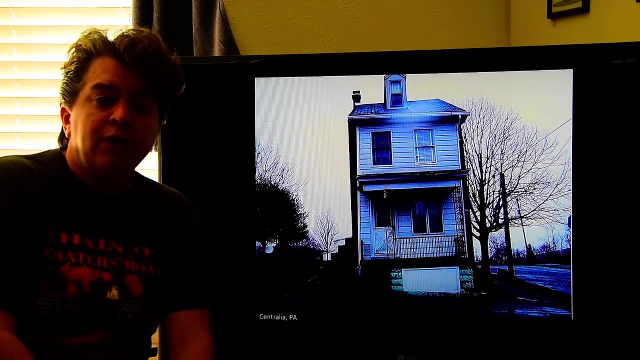 and the people didn't want that to happen, And so then the fire just grew and grew to become too big to be able to manage, And now it is simply going to keep burning until there is no coal left in that area to burn out. You might be asking: how long can that be? Well, up in.